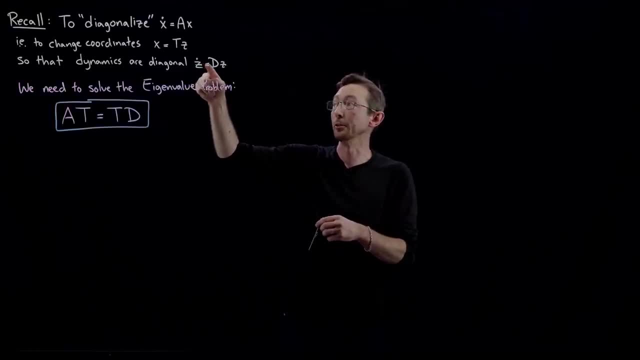 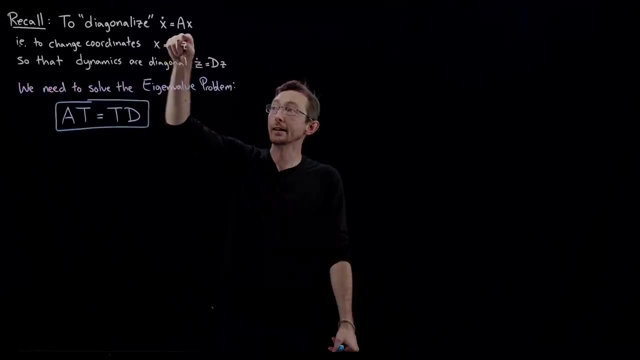 much easier to solve this differential equation where d is diagonal than this differential equation where a is kind of a generic gnarly matrix, And so we're literally trying to find this matrix T. that is a change of coordinates between x and z, where it makes my dynamics. 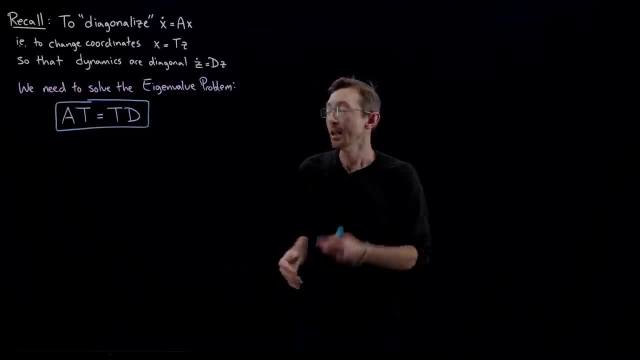 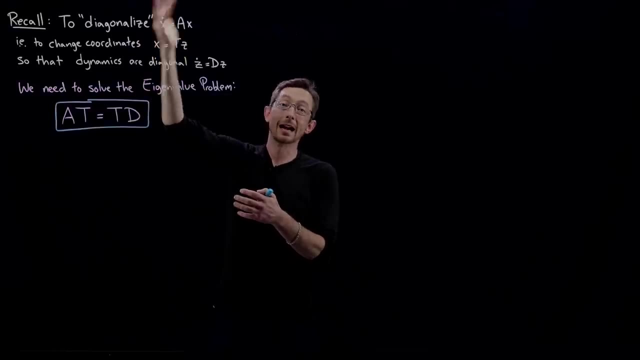 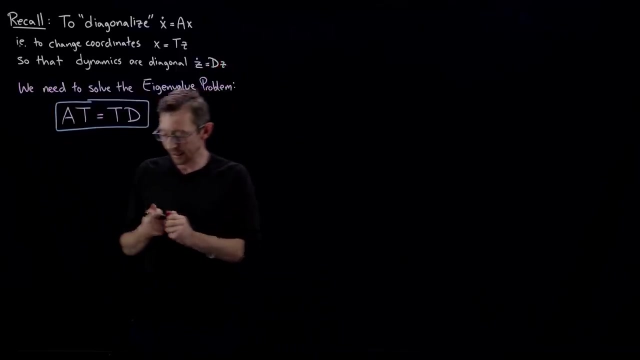 easier. We're trying to find that coordinate transformation T, And in the last lecture I derived, I showed that the matrix T that diagonalizes my system is specifically the matrix T from this eigenvalue problem, And so in this expression A is my original matrix. 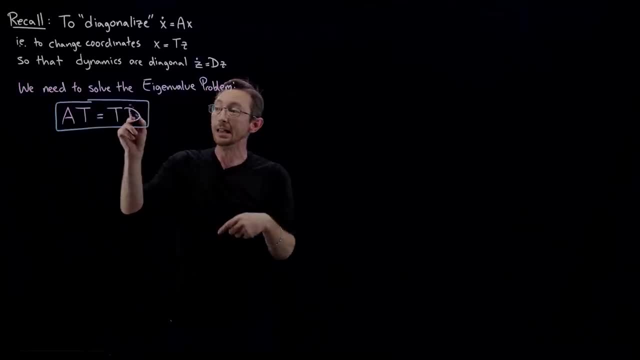 T is a matrix of eigenvectors of A and D is a diagonal matrix of eigenvalues of A. So I'll just write this out. So these diagonal entries, diagonal entries, are eigenvalues. This is a German word I'll tell you about in a minute: eigen. 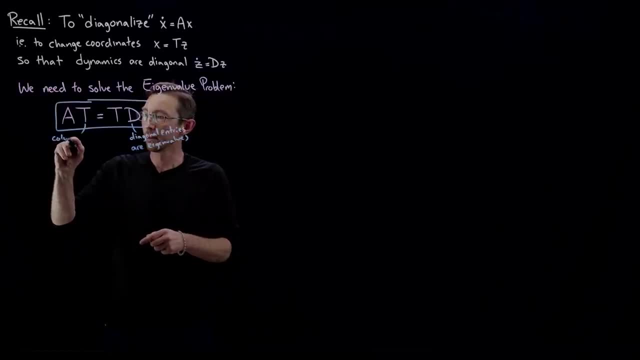 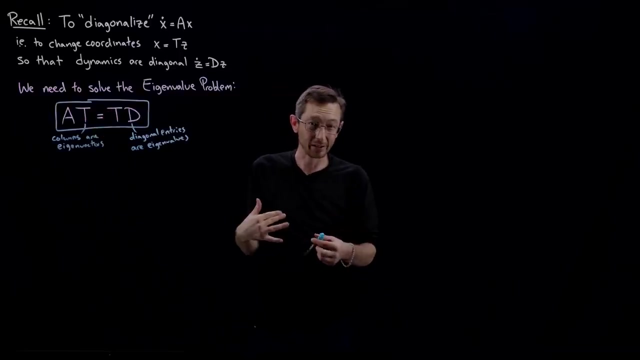 And the columns of T are my eigenvectors And so instead of thinking about this as a matrix eigenvalue problem, it's sometimes a little easier to just think about finding individual eigenvectors and eigenvalues one at a time, So kind of columns of T and entries of D, you know, finding those one at a time. 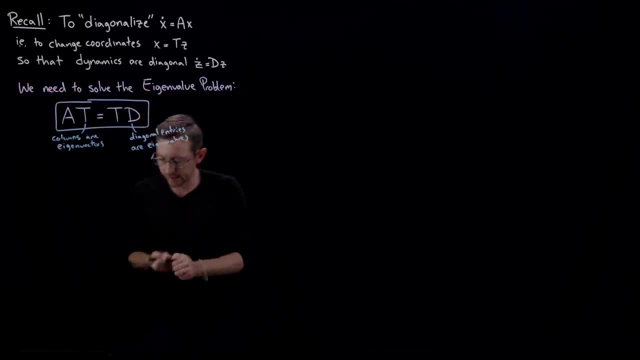 And so the way I'm going to write that, that is this: AX equals lambda X. Okay, so the German word eigen literally means like special or characteristic, And actually in German it means latent or characteristic. I'm going to write this down: 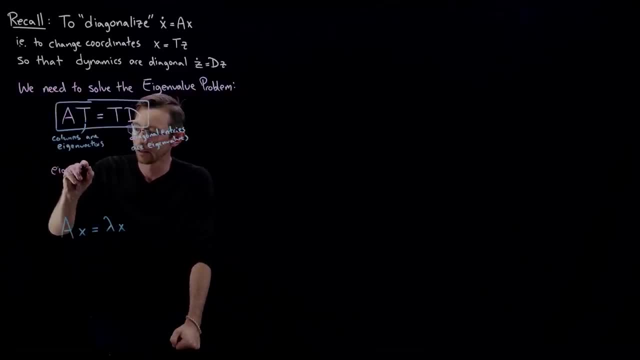 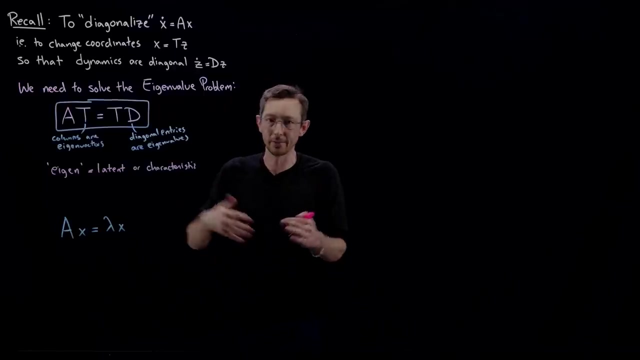 So like eigen means latent or characteristic. What that means is kind of like the essence of it's, the essence of something. So if you like, boil off everything else. the latent or the characteristic part is what's going to remain, the eigen part. 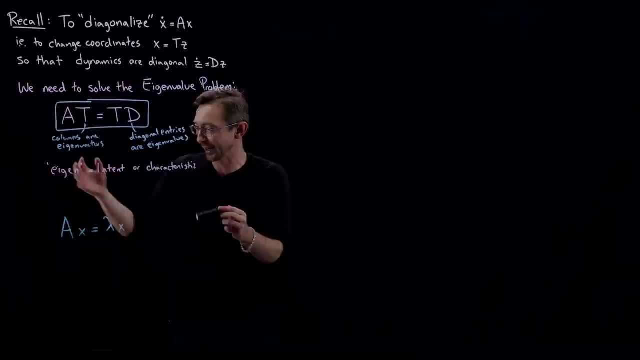 So you'll notice my channel is called Eigen Steve. I'm Eigen Steve, Eigen, just. and also, I guess when I think of eigenvalues and eigenvectors I'm thinking these are kind of special values and special vectors. I'm going to define what I mean by special in a minute. 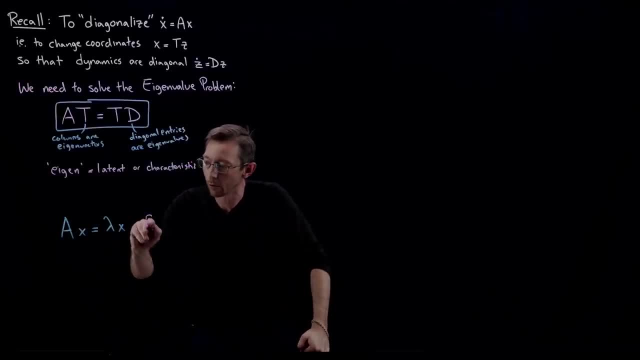 But again, I'm going to write this down. So I'm going to write this down: AX equals lambda, X for special vectors, X and for special values: lambda. And that's kind of. what I mean is that these X are going to be eigenvectors. 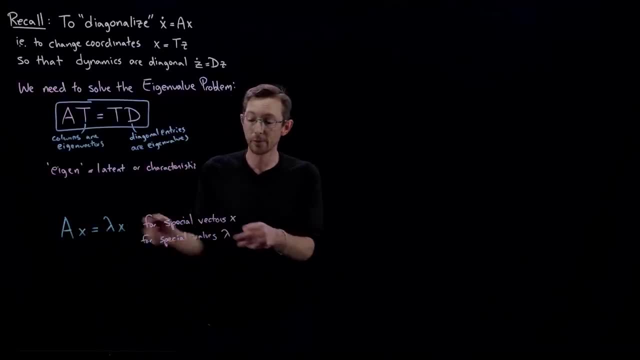 Those are special values, special vectors where this is true, And lambda are special numbers, where this is true. Not all lambda, Not all lambda are going to satisfy this equation And not all vectors X can satisfy this equation. Only very special vectors X and special vectors lambda can satisfy this. 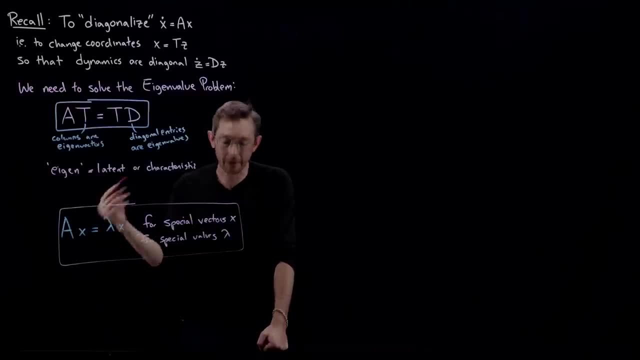 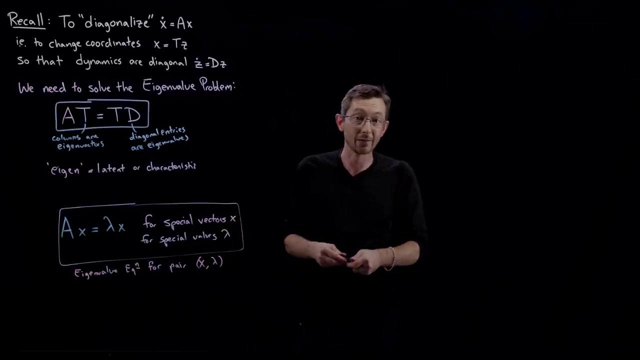 Good, And this is the eigenvalue equation for a single pair: X comma lambda. So this is the eigenvalue equation for a specific pair, for a pair of eigenvalues and eigenvectors- X comma lambda. So they always come in pairs And eigenvector always has an eigenvalue associated and an eigenvalue always has an eigenvector associated to it. 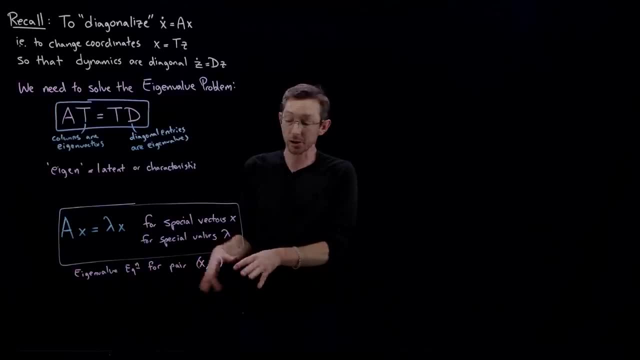 Okay, so this is what I'm going to talk about today in this lecture. I'm going to give you some numerical- is not not numerical by hand- examples. We're going to actually compute these special vectors, X and special values lambda for a particular, a matrix that I'm going to write down. 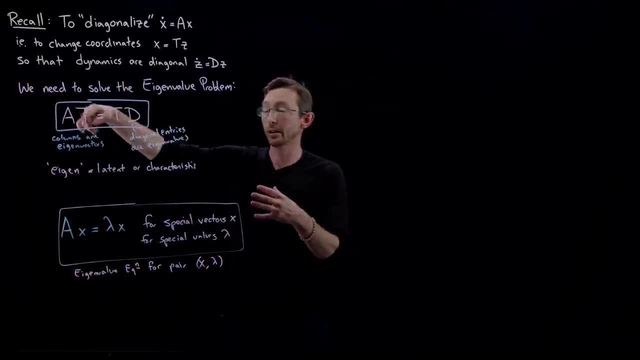 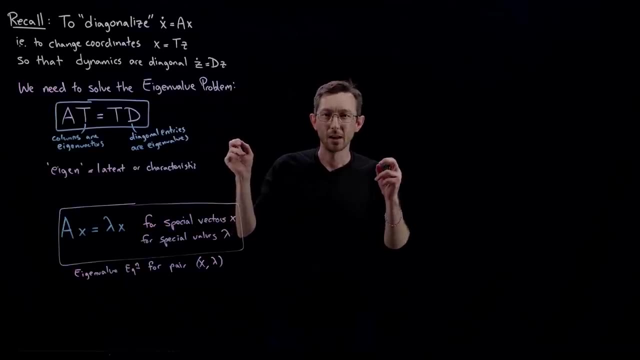 And then we're going to talk about how to compute these in general for an arbitrary matrix A. now what I want you to notice here is that my definition of special is is pretty easy to understand. I guess is what I want to say. what I mean by 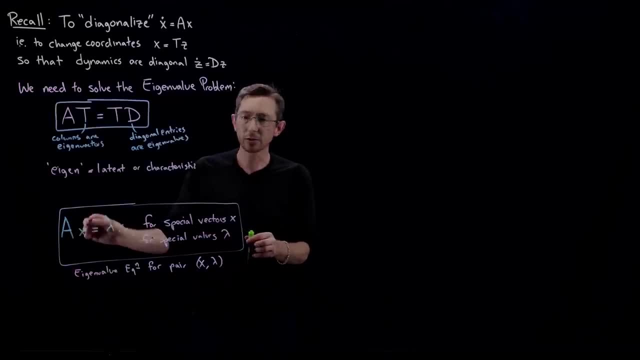 special is that there are special vectors X that when I multiply them by this matrix a, the direction of X doesn't change. it just gets scaled up or down by lambda. so what I mean here is that multiplication by a matrix. I usually think of that as a coordinate. 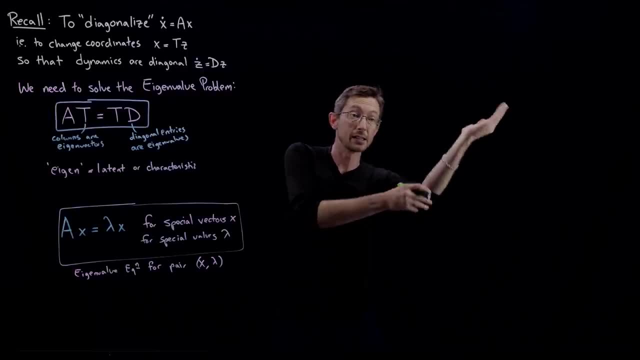 transformation. so vectors, when you multiply them by matrices, typically they'll, you know, rotate and maybe stretch and they deform. so you can take all of your, your vectors in X and when you multiply them by a it's going to kind of rotate and deform generically those vectors, and there are some very 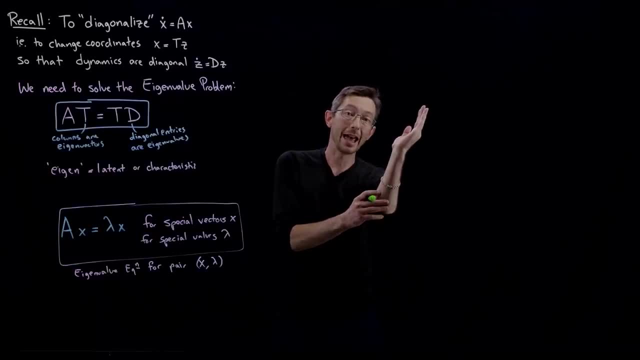 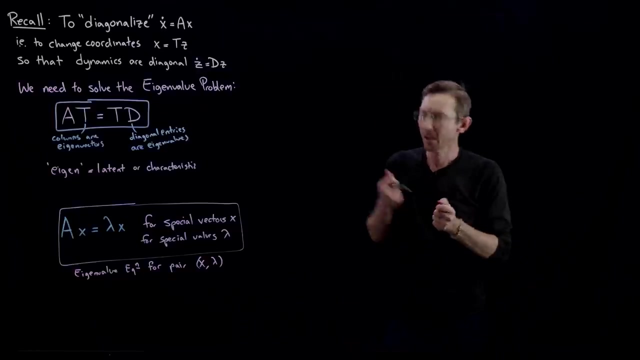 special vectors X, that when you multiply them by a they don't rotate, they just get longer or shorter. and that's what i mean by these eigenvalues and eigenvectors. so that's the example i'm about to show you. maybe i'll move my notes over here so i have some room. so let's just do an example to get. 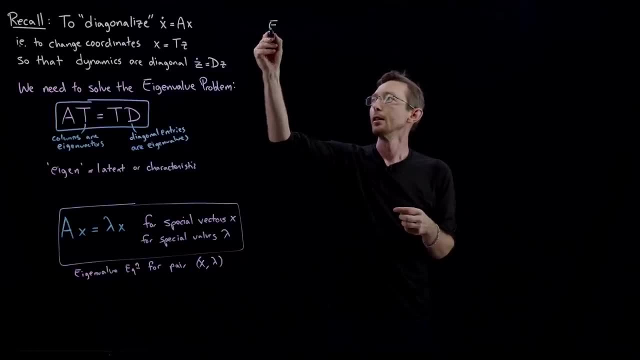 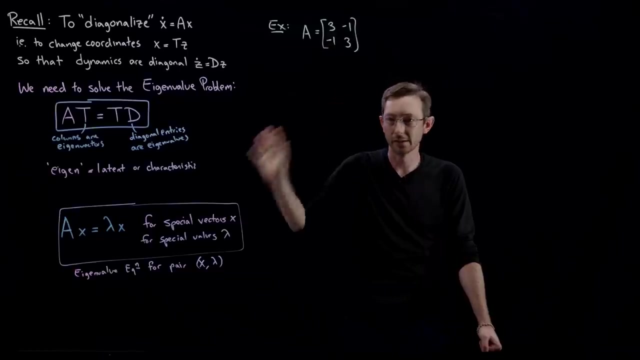 some intuition and then we'll talk about this in the generic case. so an example, a matrix. i'm going to pick an, a matrix that is 3 minus 1 minus 1, 3, 3 minus 1 minus 1, 3, just a little simple, 2 by 2 a. 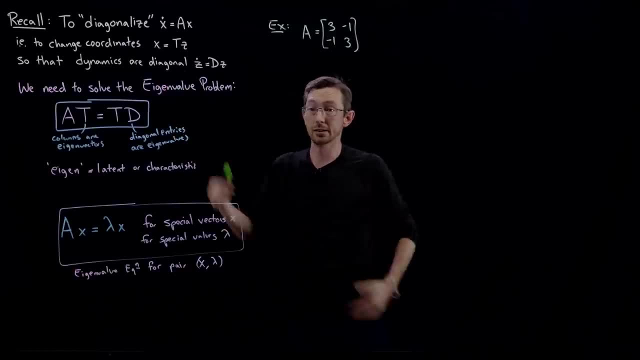 matrix, but it's not diagonal, so it's going to be difficult to, you know, do solve differential equations with this a matrix. and so what i'm going to do is i'm just going to try, like a random x vector, i'm going to just pluck an x vector out of a hat, multiply it by a and see if it satisfies. 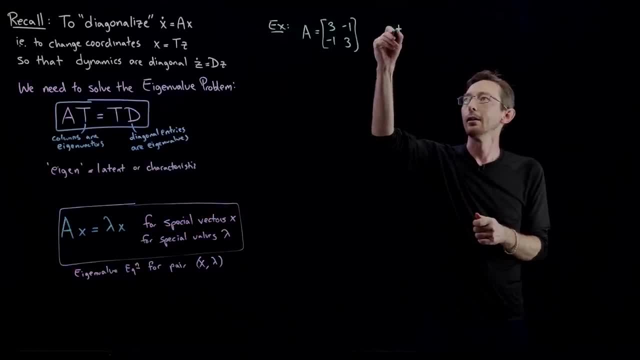 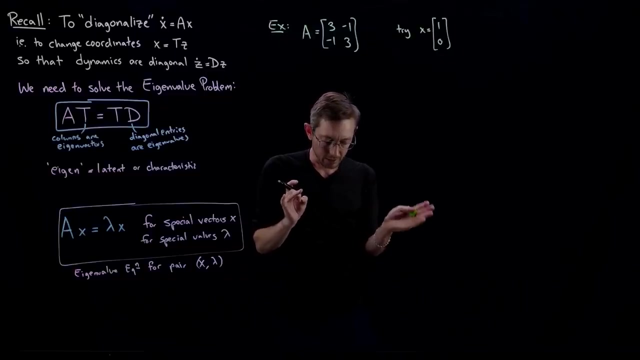 this equation, okay, so we're going to try. let's try: x equals, you know, 1, 0. that's kind of the easiest thing we can try. let's try: x equals 1: 0. and i'm trying to think of how i want to draw this, because i'm going to draw you a picture. 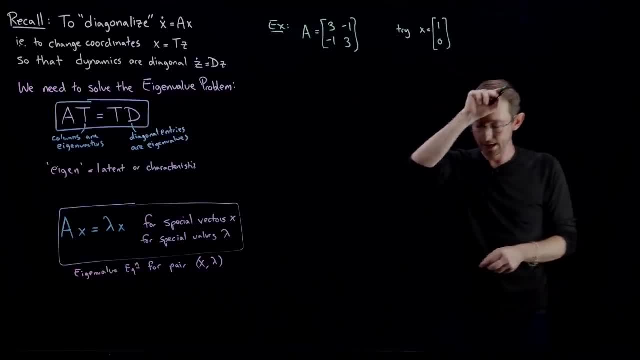 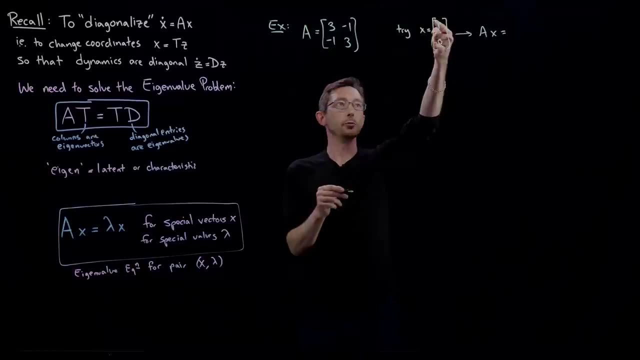 but let's, let's try. x equals 1: 0, then a x, a x is going to equal. i literally can just multiply a times x and it's going to be equal to a times x, and it's going to be equal to a times x. 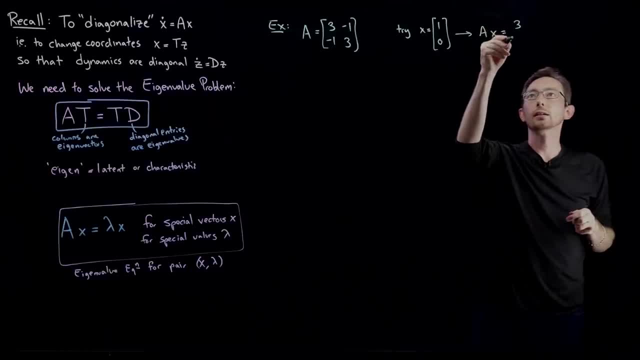 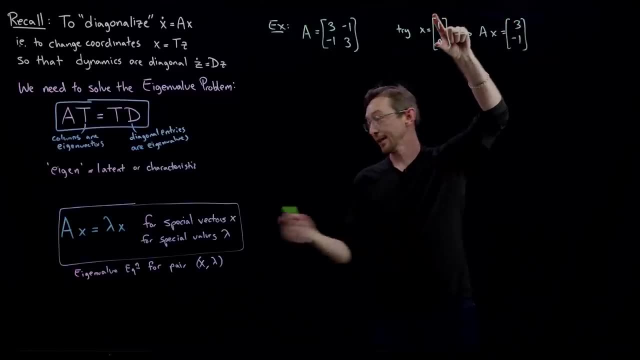 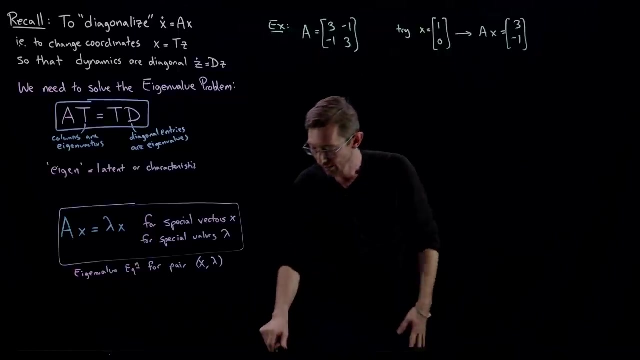 and it's going to be 3 negative 1. this is 3 negative 1, okay, and clearly you can see that a times x is not just x times some number, it's not just x longer or shorter. they point in different directions, completely different directions. so i'm going to draw a picture, um, and i want to be very 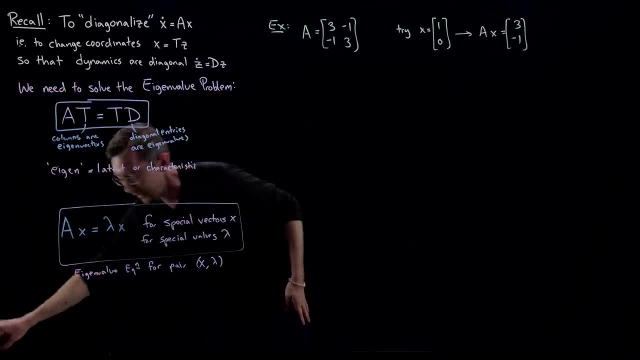 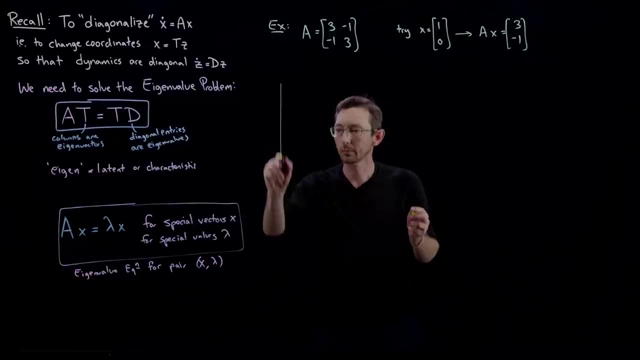 careful about what colors i use, otherwise this is going to get impossibly messy. so let's say, i have my, my x 1 and x 2 axes here and my first test vector. maybe i'll draw some ticks. you know, one, two, three, four, five, six, seven. one, two, three, four, five, six, seven. i could do this in a 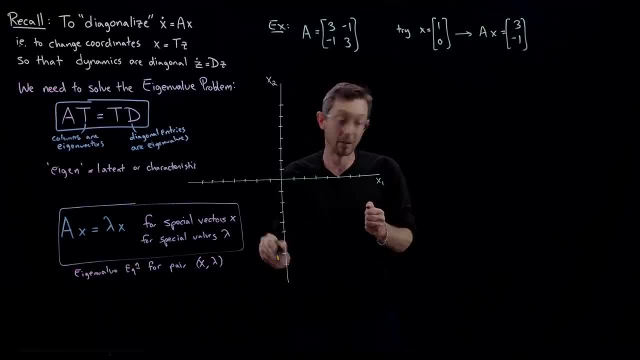 computer, but i think it's way more fun, uh, to do it by hand. um, this is going to be a little bit more. this is how i always think about it. so what i literally did here is: i took this test vector, um, this test vector x, this vector 1 comma 0. you know it's 1 in this direction, 0 in this direction. 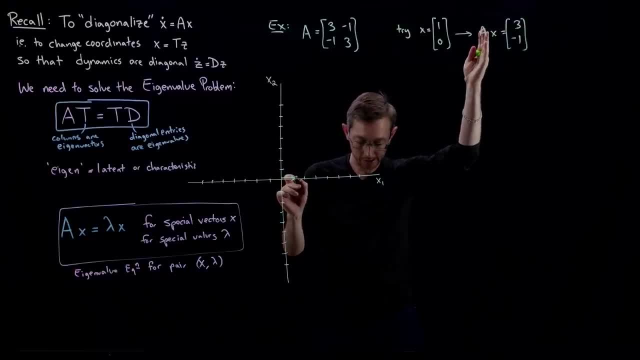 and i multiplied it by a and i got something that was 1, 2, 3 negative 1, so i got something that points in a completely different direction. this was x and this was a x. they point in completely different directions, so they can't possibly be eigenvectors, or i you. 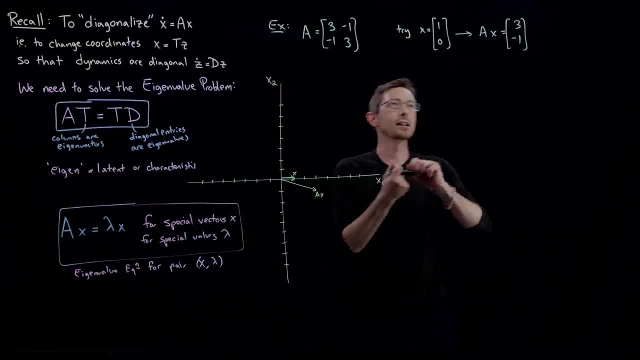 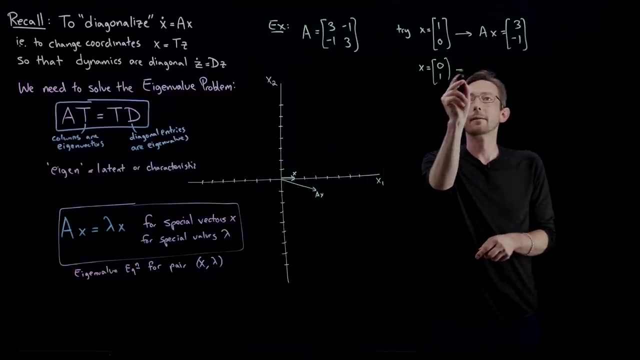 know eigenvectors of this system. good, um, let me try one other example, just you know to to illustrate. let's try: x equals uh, 0, 1. so now, instead of pointing in the x direction, it's going to point in the kind of x, the x 1 direction will point in the x 2 direction. um, again, i can multiply this by: 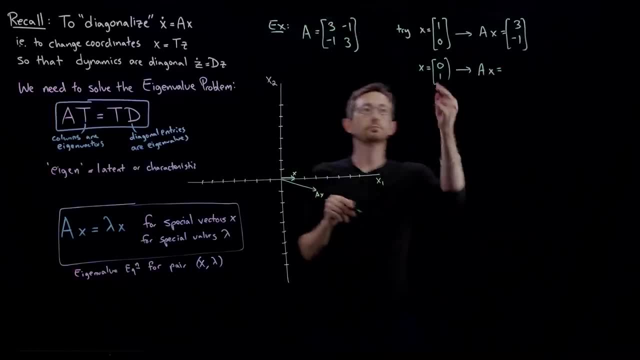 a and i get a x equals. now it's going to be negative 1: 3. so that's negative 1: 3. that means that i'll pick a different little color here. i'll just do yellow, because they're kind of pretty similar: yellow and green. 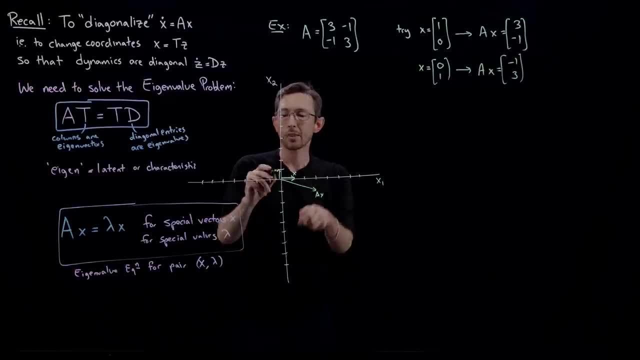 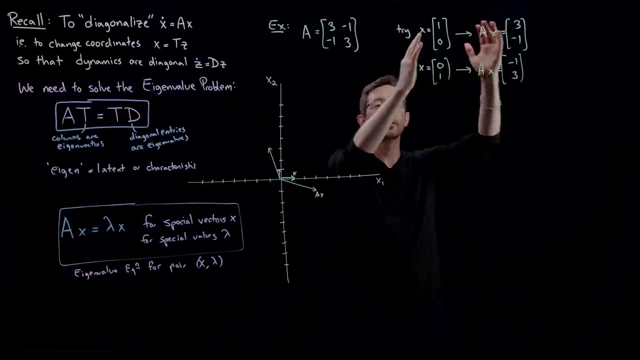 so now this little uh vector here multiplies to negative 1, 1, 2, 3 again these are pointing in different directions. so my vector rotated after multiplication by a, and so neither of these kind of principle x1 or x2 directions are eigenvectors of my A matrix. These are not. 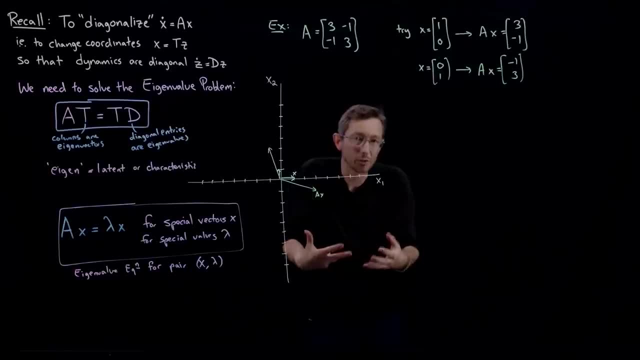 eigenvectors, So there are special vectors. I haven't convinced you yet, probably, that there are in fact, these magic vectors where this is true. So what I'm going to do is I'm actually just going to write them down. I'm not going to derive them yet, I'm just going to write them down. 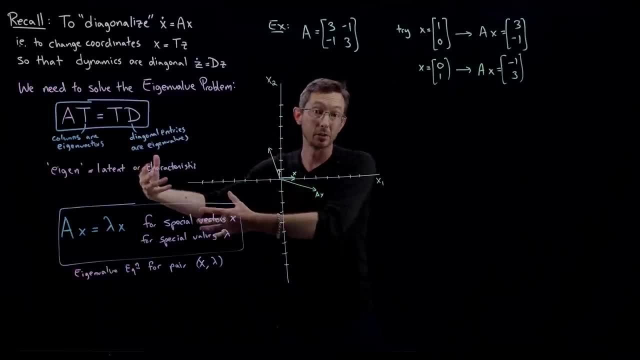 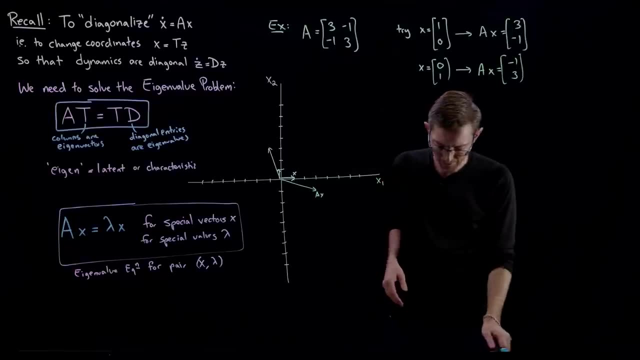 show you that they have this property and then I'm going to show you how to solve for them if you had this, A matrix. And I'm going to do this in blue and pink. So the first special value is- I'm going to claim that the first special, and sometimes I call my eigenvectors xi, Sometimes I 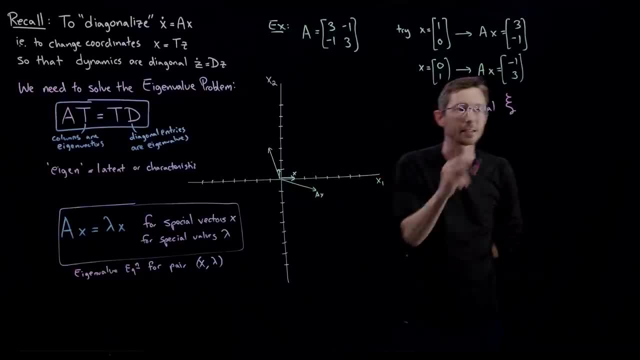 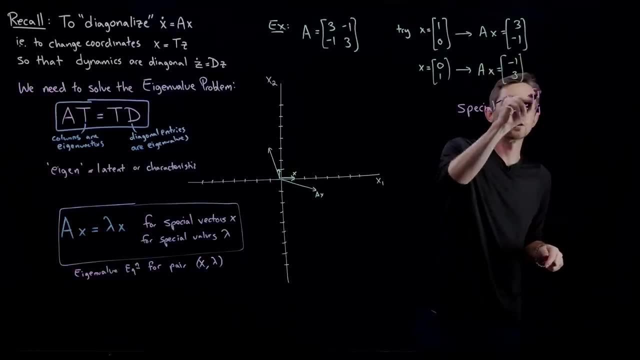 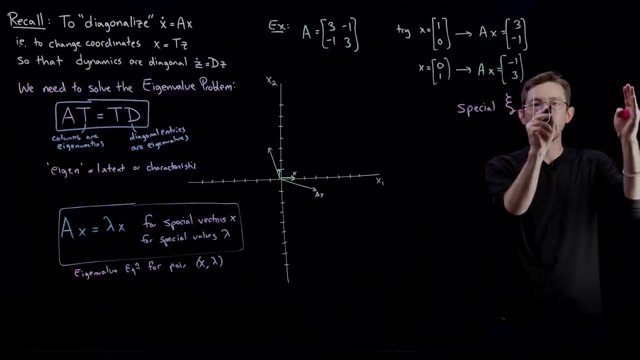 like to use my fancy pants xi vector here, because I really like xi. Xi and I are old friends And the first eigenvector is going to point in the 1, 1 direction. Okay, this is I claim an eigenvector. Let's see if this is true. So I'm going to multiply this by A. 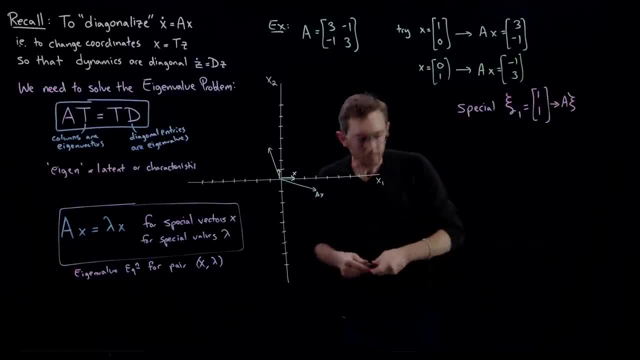 I'm going to take A times xi. What happens when I multiply A by 1, 1?? I get 3 minus 1 is 2, and minus 1 plus 3 is also 2.. So this equals 2, 2.. And lo and behold, this actually is in the. 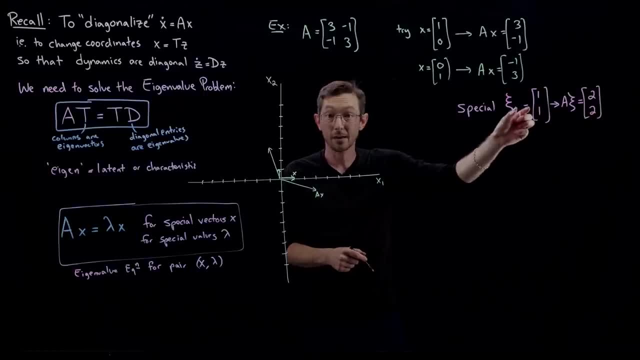 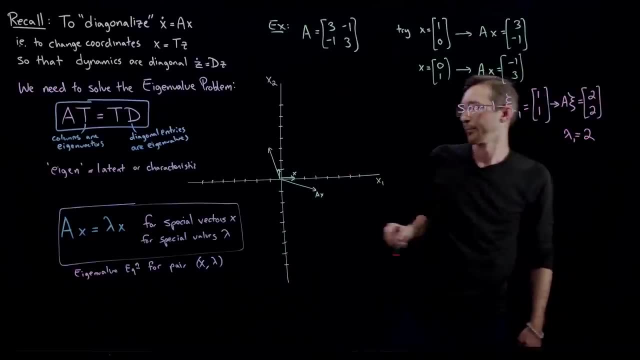 same direction as xi. It's exactly 2 times xi. So I'm going to take A times xi And I'm going to stretch xi by a factor of 2.. So this is my lambda: 1 equals 2.. Okay, so A times xi is equal to 2 times. 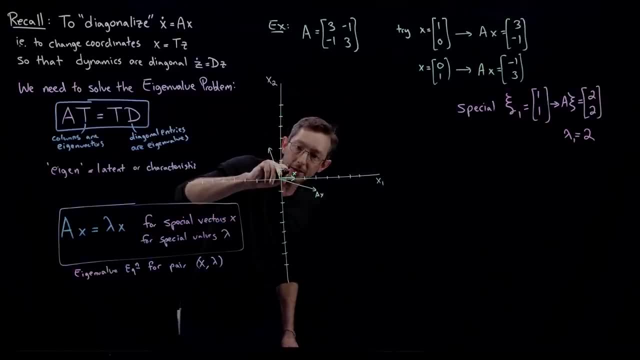 xi. That's good. So I'm going to draw this picture. So this vector here in the 1, 1 direction, this xi is an eigenvector, because when I multiply it by A I get a vector in the exact same direction, A times xi. 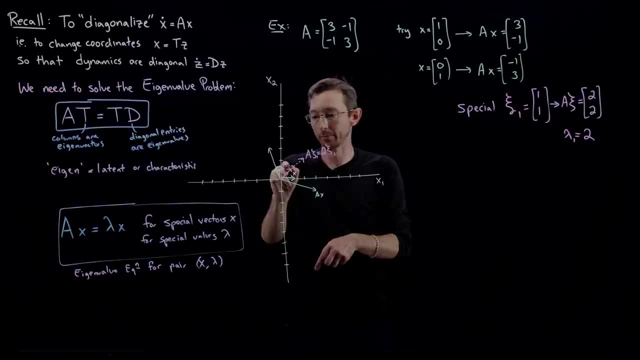 So this was xi 1. So that's really really special. That's what I mean by an eigenvector. They are special kind of magic directions where if I take a vector in that direction and I multiply it by A, that vector stays in that direction. Very, very interesting, Very very important. 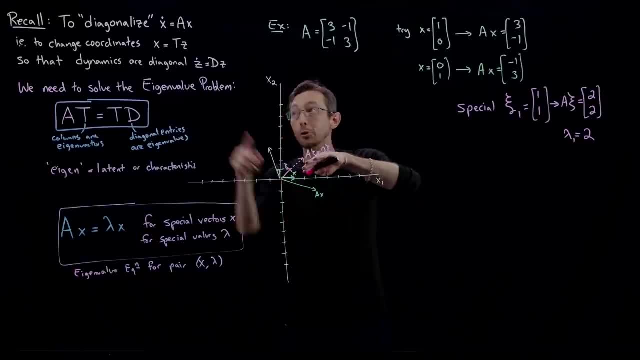 And you can almost picture how those special directions where, if I multiply by A things, stay in that direction. That's how I'm going to decouple my dynamics, because in these directions my dynamics are completely decoupled in this direction and in the other. 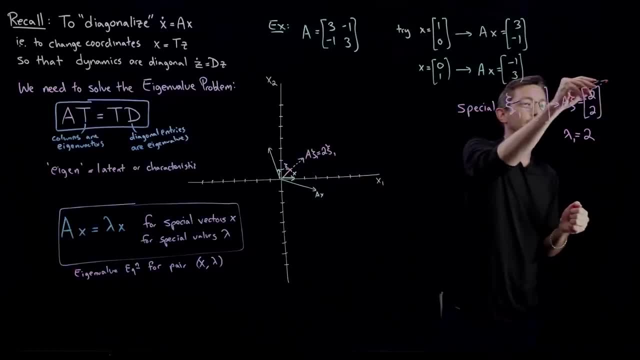 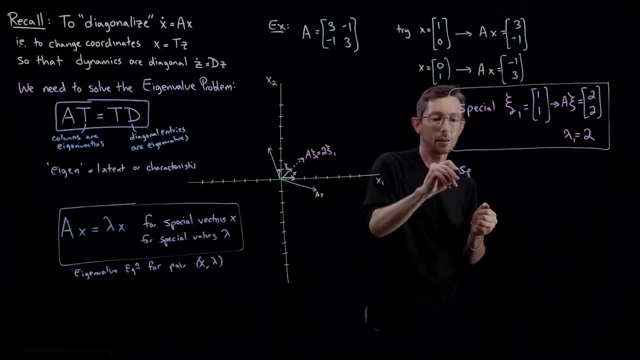 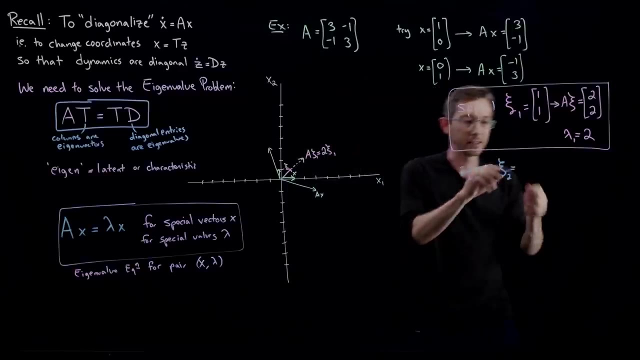 direction. I'll get back to that later. So that's one special eigenvector xi. The next special eigenvector, my next special, xi 2, I believe it's going to be like 1 minus 1 or something like that, So it's 1 minus 1.. I've had a lot of experience with eigenvalues and eigenvectors. 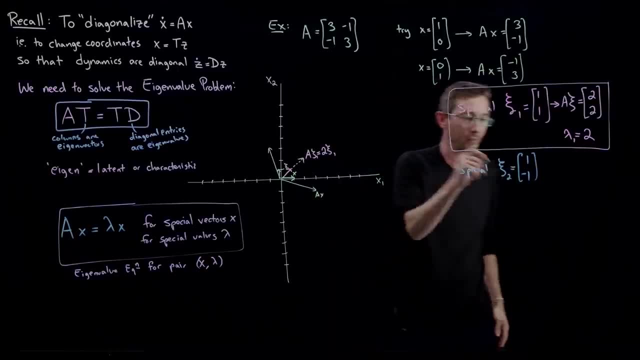 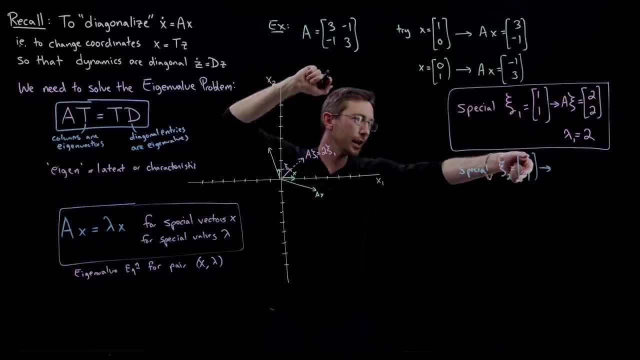 Almost. you can read these off of a 2 by 2 matrix, but you'll get there. if you can't do that already, Let's multiply A by this now, And so now I'm going to multiply it and I get 3 minus minus 1 is 4.. 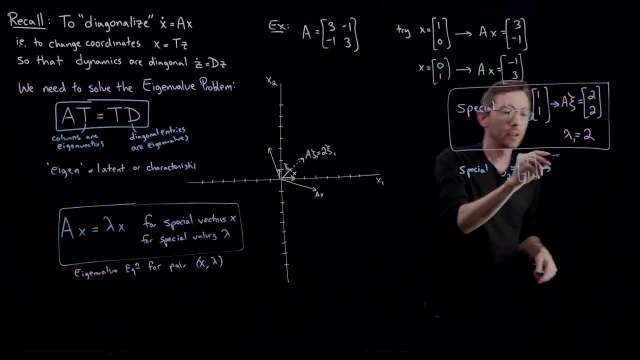 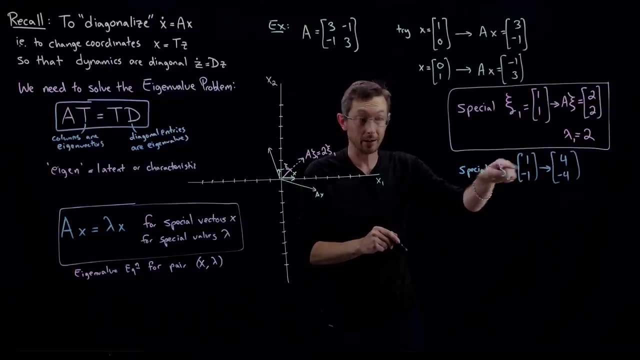 And minus 1 minus 3 is minus 4.. So I get 4 minus 4.. Again, this is just a constant scaling of xi 2. Sorry, I should have written that this is A times xi 2. And that's what this 4 negative 4 is. 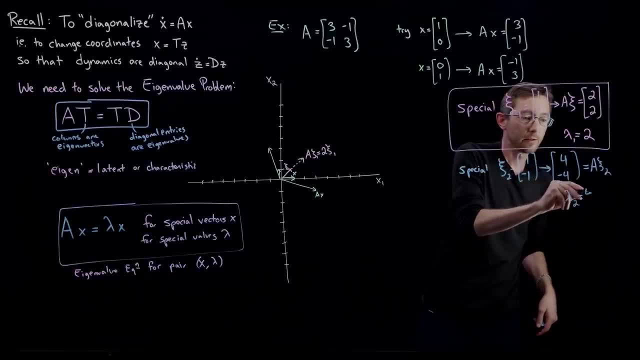 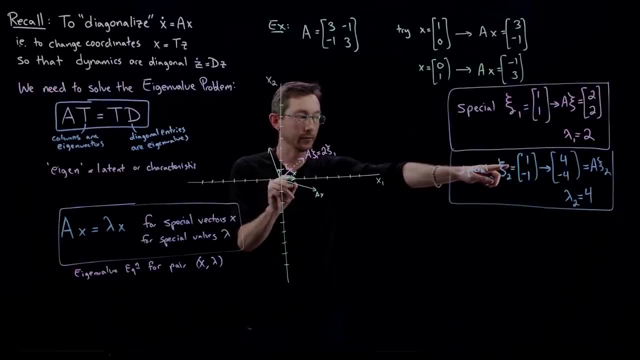 And so my lambda 2 equals 4.. Okay, So I can again draw this one. So I take a step 1 in the first direction and minus 1 in that direction, That's xi, 2. And if I multiply it by A, I take 1,, 2,, 3, 4 steps. 1, 2,, 3, 4 steps. 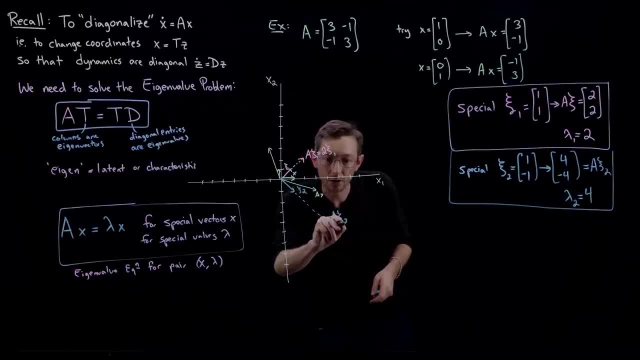 And this is A times xi 2.. And that just equals 4 times xi 2.. So there are in fact these very special kind of eigen directions, these eigenvectors x. I call them xi 1 and xi 2 here. 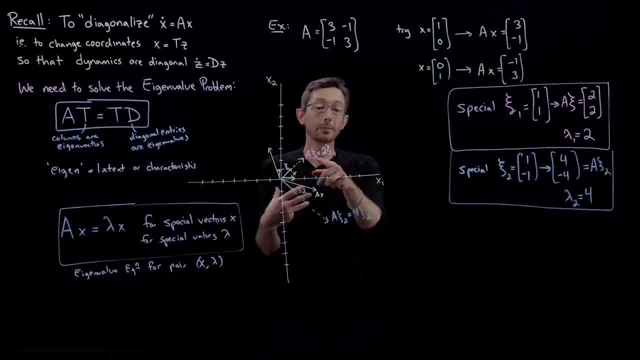 These pink and blue directions where, if I multiply those very special vectors by my A matrix, I get a vector in the same direction. in the same direction that's just scaled by lambda- In this case, lambda 2.. In this case, lambda 2.. And in this case, lambda 3.. And in this case, lambda 2.. And I 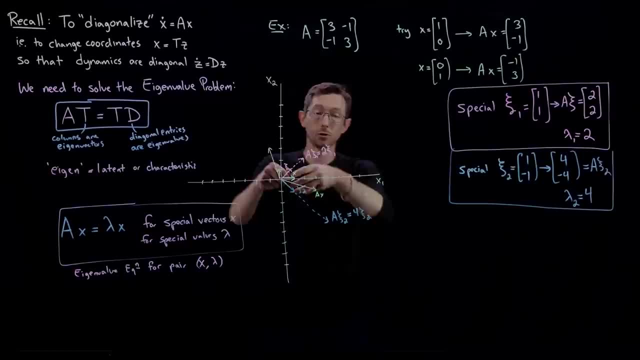 to four. okay, And I think I showed you and I convinced you. if I just randomly pick a vector and I multiply it by a, it's going to rotate, It's going to go into a different direction. So not all vectors x are eigenvectors. Only very special vectors are eigenvectors that have this. 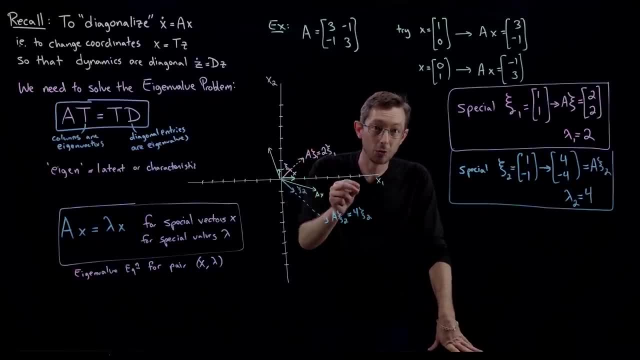 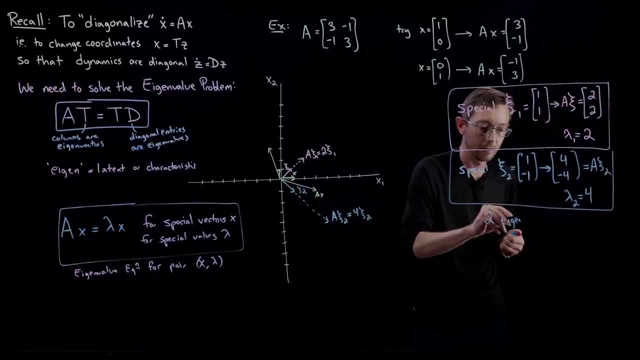 property. Good, okay, So there's exactly two eigenvalues and two eigenvectors for this, two by two system. I'm just telling you that's true right now. We'll see that that's true in a minute. okay, There's exactly two. There's two kind of eigenvectors and values. Good, And again. 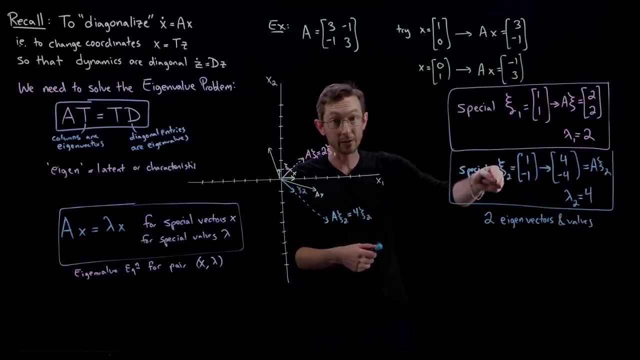 they come in pairs. This is the eigenvalue corresponding to this eigenvector. And similarly, this is the eigenvector corresponding to this eigenvalue. They come paired up. That's why I color-coded them. Okay, good, So hopefully this builds your intuition. Now what I'm going. 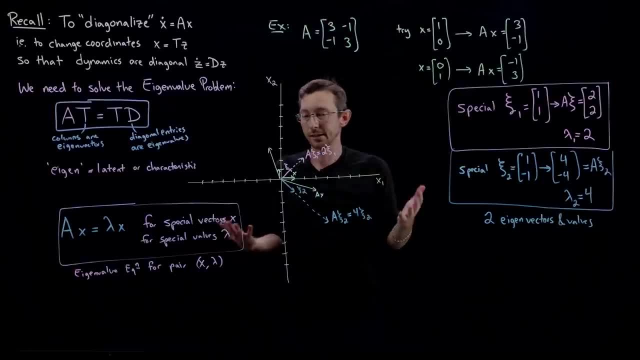 to do is. you know, this is just one example for one AMA, That's not that generic. So now what I'm going to do is I'm going to show you how to solve for these eigenvalues and eigenvectors for a generic matrix. Okay, so now we're going to go and how to 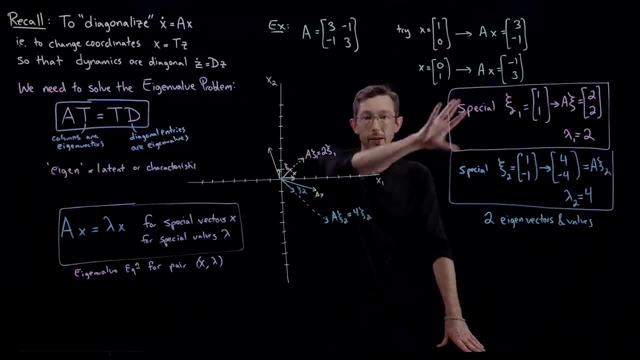 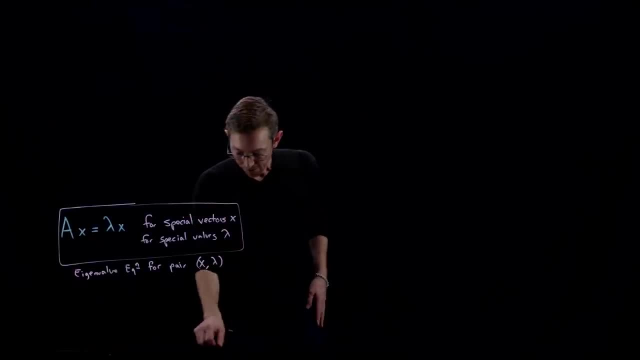 do this in general. So I'm going to erase all of this and then we're going to work that out. Okay, so I've given you some examples of eigenvalues and eigenvectors. Now I'm going to show you how to solve for them in general. Someone gives you. 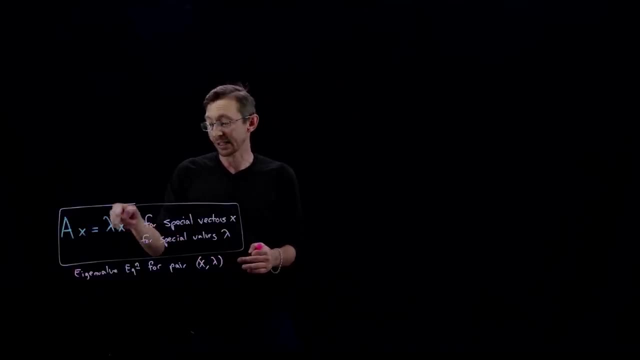 you know a random A matrix, You're going to be able to figure out what are the special X and lambdas that are eigenvalues and eigenvectors. So I'm literally going to take this equation here and I'm just going to rewrite it a little bit. So I'm going to say that and I want to give myself 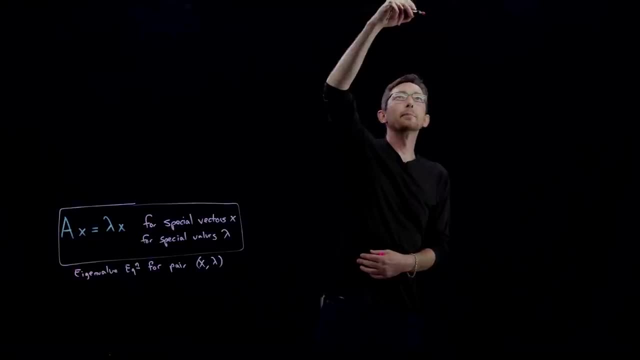 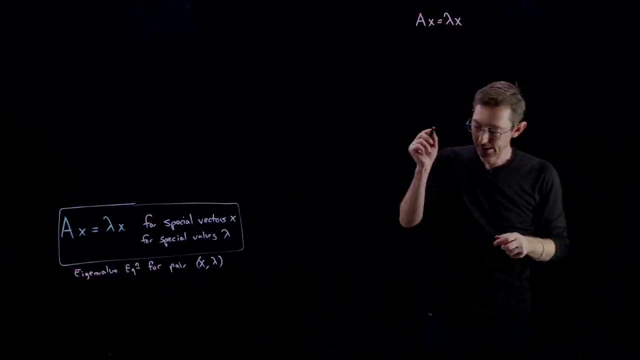 a little space here. I'm sure I'm going to need it. So I'm going to say that AX equals lambda X. You can always do this with matrices. You can say that lambda just a number times a vector X is the same as that number lambda. 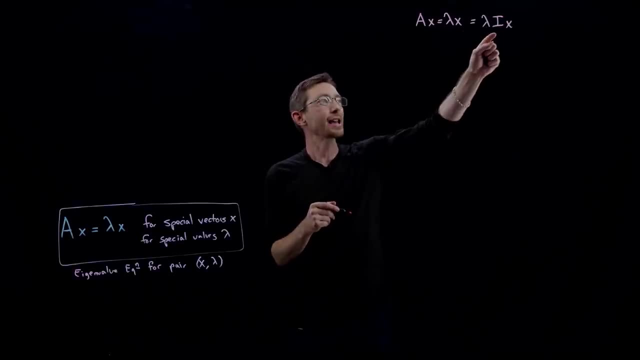 times the identity matrix times X, Because any vector X is just the identity matrix times that vector X. So I can, little you know, pop in a matrix- I here, If you are confused by that pause, and you know, write this out with an identity matrix times X and convince yourself that that 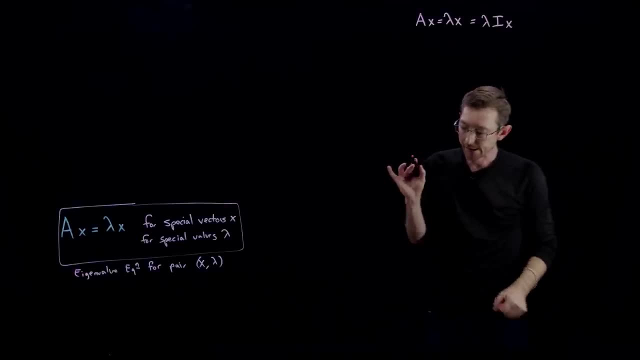 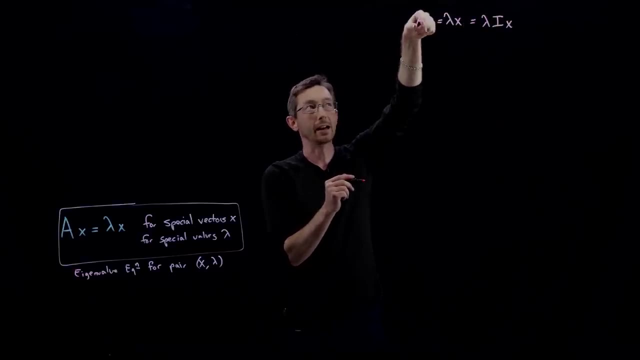 is exactly just X. It's totally fine, And so essentially you're going to be able to solve for this. So essentially now I can move this. The reason I'm doing this is because now I can move this over to the left-hand side and I have matrix A, matrix lambda I times vector X, So I can move. 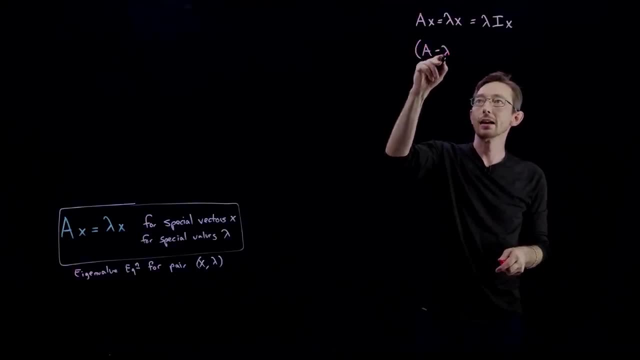 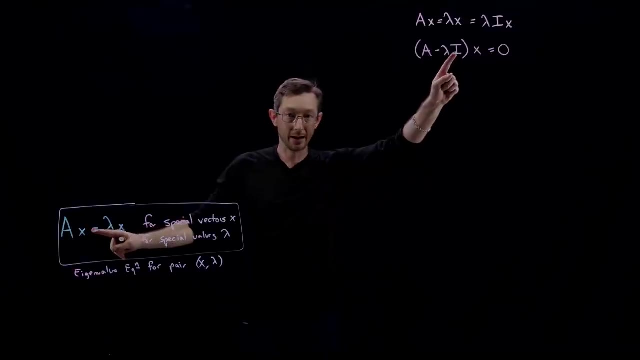 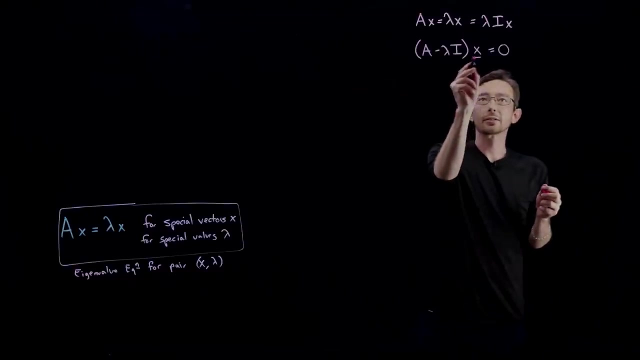 this over to the left-hand side and say A minus lambda times the identity matrix X equals zero. This is equivalent to my eigenvalue problem here. This is an equivalent way of writing it. And again, you know X is a vector. It's a vector of zeros. A and I are matrices. I'll just put them here so you remember. 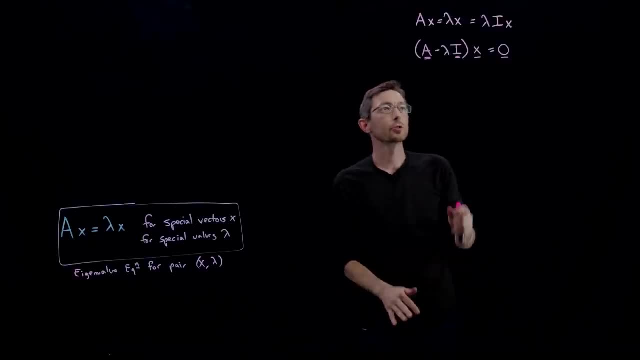 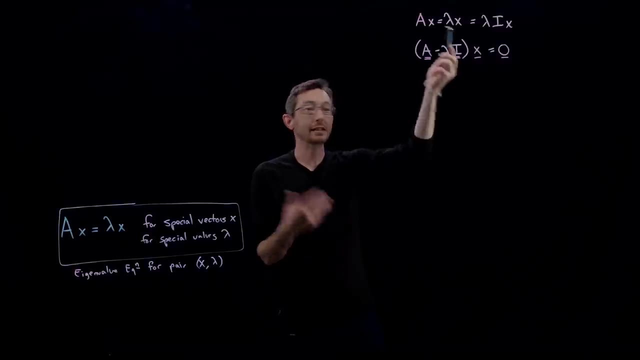 And lambda is a number, And so what we're trying to do is we're trying to find X and lambda- pairs of X and lambda that satisfy this equation. Now you might imagine: well, this is easy, I'll just make X equals zero, And then this is always true. That is technically, mathematically true. 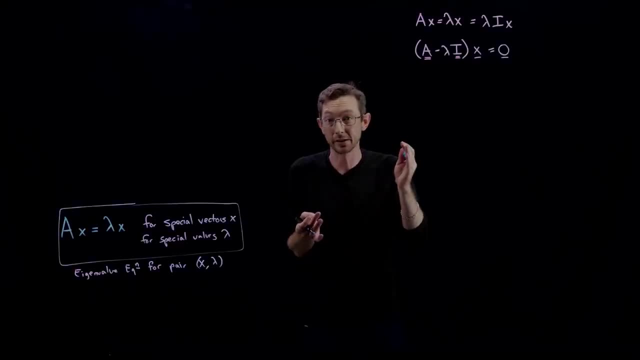 but that's kind of boring. It's not really a vector. X equals zero is not a vector, It has zero length. And so I'll just put this here. And then this is always true, And so I'll just put this here And I'll just write down, you know, case one: X equals zero is kind of a solution. 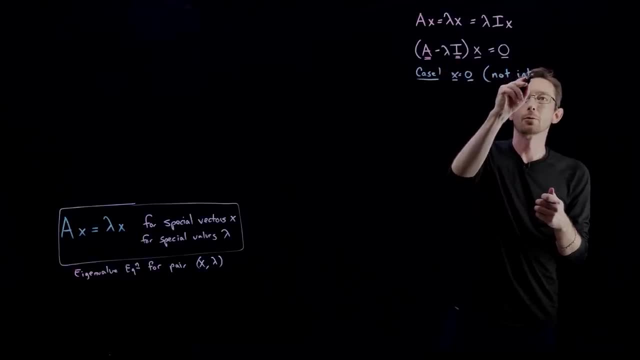 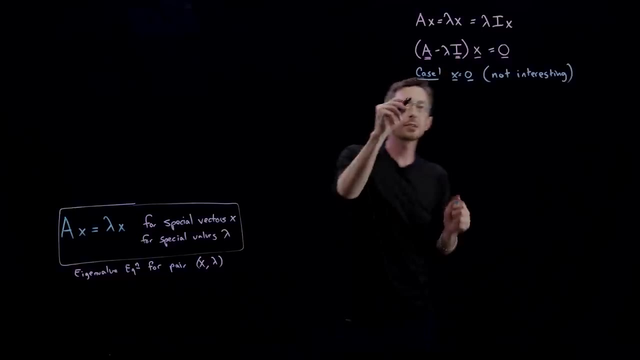 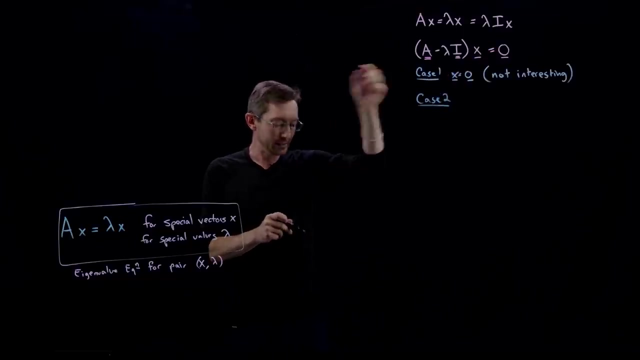 but it's not very interesting. It's not what we're looking for Interesting. These are not the droids you're looking for, Okay, not the eigenvectors you're looking for. Case two is more interesting, So case two. the other way that this can be equal to zero is for X to not be zero. 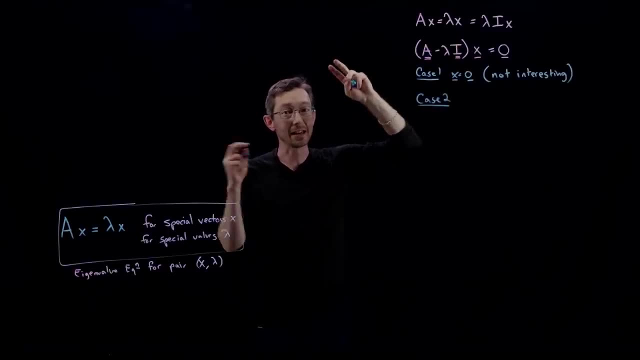 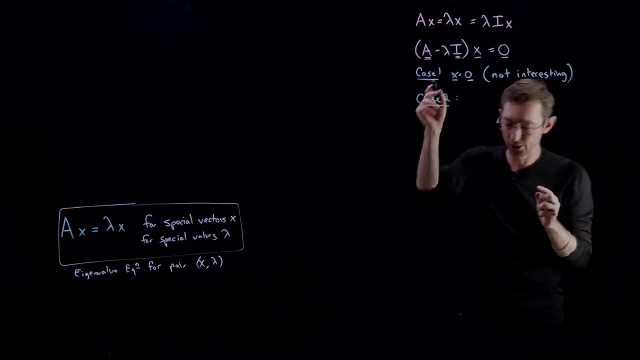 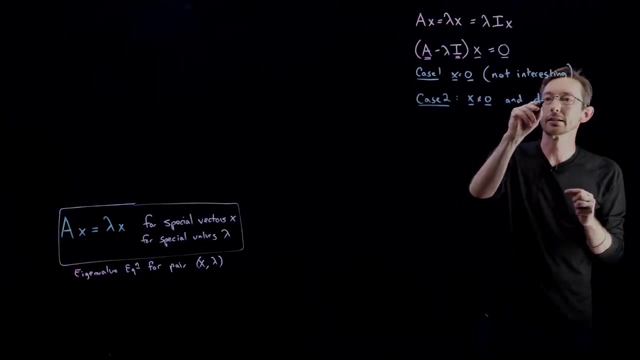 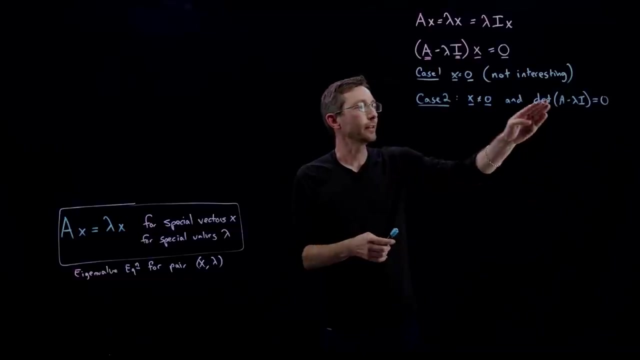 and for this matrix to be what's called singular meaning. it maps certain vectors to zero. Okay, I'm going to write this out and then I'm going to explain it. So case two is where X is not zero and the determinant of A minus lambda I equals zero. If the determinant of A minus lambda I 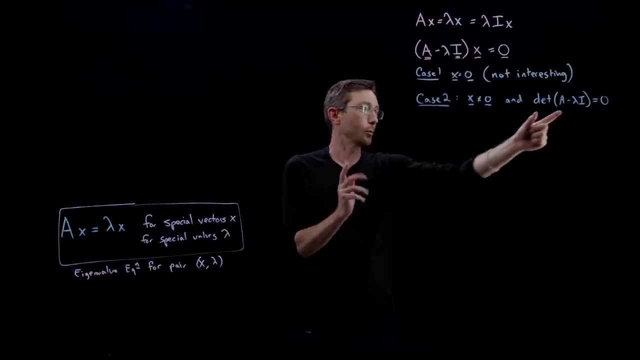 equals zero. that means there are some directions where this matrix is not zero. This matrix will map those directions to zero. Okay, I'll draw you a picture later. Just take my word for it for now. That's what this means is that if I have a matrix A minus lambda, I, with 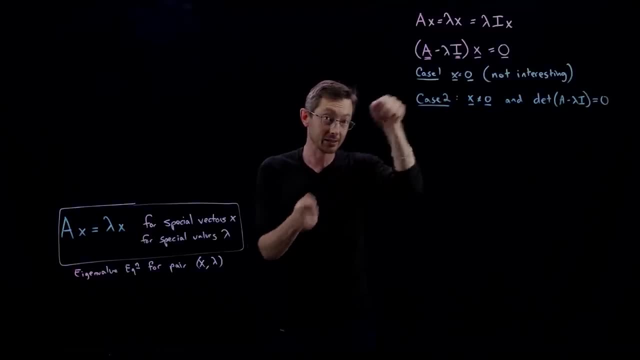 determinant zero. there are certain subspaces, certain directions that if I multiplied them by that, I would get zero, which is kind of what I'm looking for. I'm looking for an A minus lambda I, where there's directions that map to zero. Okay, so that's kind of what I'm looking for. 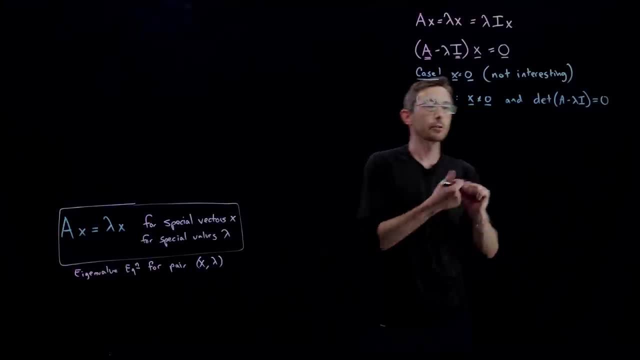 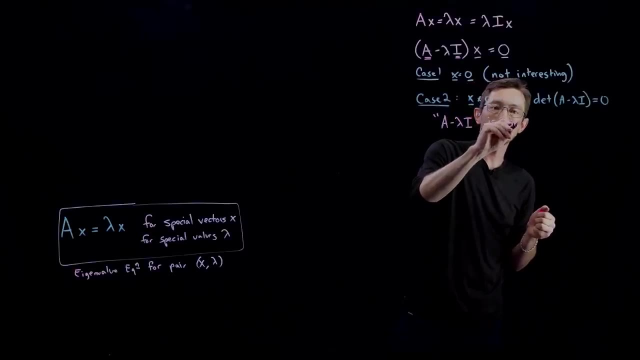 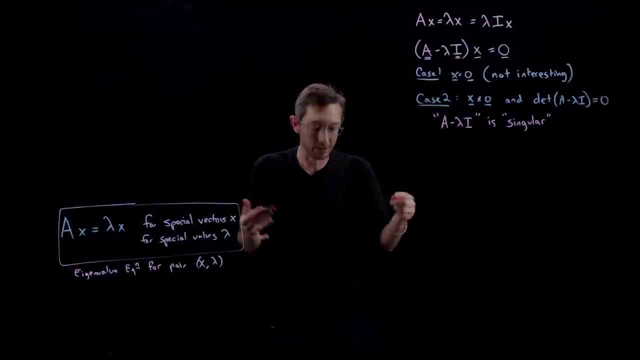 Okay, so that's kind of what I'm looking for In this case. we call it a matrix: A minus lambda I. We call this singular. We say A minus lambda I is singular. I put my air quotes on the wrong thing: A minus lambda I is singular. That's just the words we 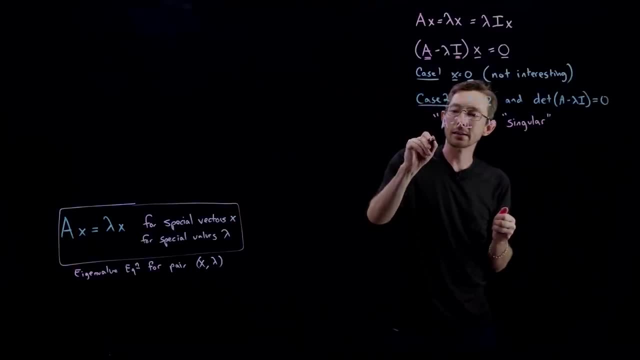 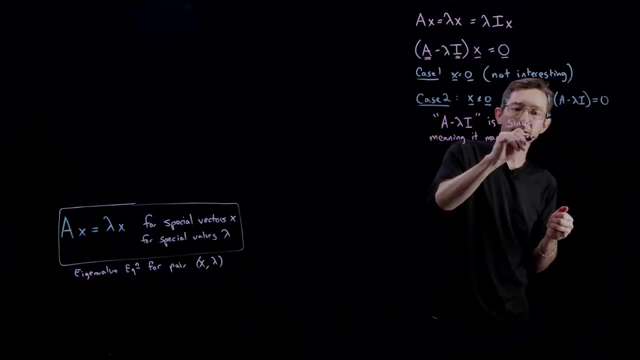 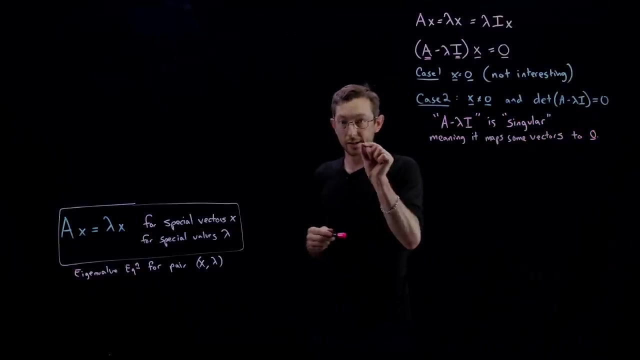 use in math to describe this, and that means meaning it maps some vectors, some vector, some vectors, to zero, Okay, to the kind of zero origin point. I'll convince you that this is true in a minute, Just bear with me. And so this expression here, this determinant of A minus lambda, I. 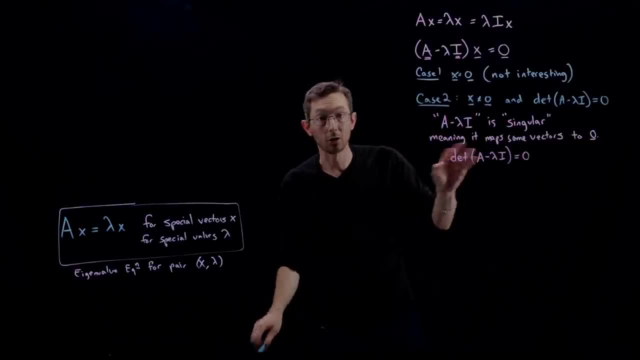 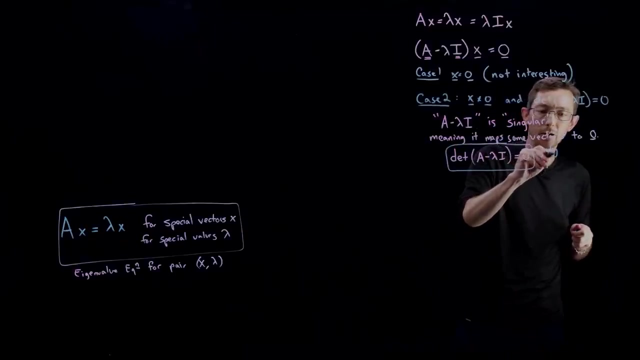 equals zero. this is not true for all lambda. Remember, I showed you in a couple of lectures ago that this is actually the characteristic polynomial of our differential equation. So this is a polynomial equation, a polynomial equation in lambda, And the roots are my eigenvalues. 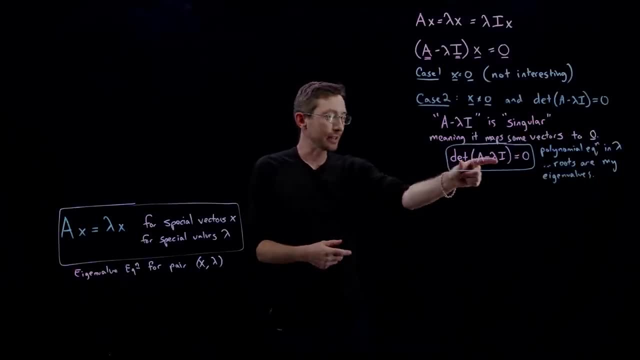 my Eigen values. So the first thing I do is I- literally this is something I can write down. I can write down A. I can write down lambda, I. I can write down this determinant, Set it equal to zero. I get a polynomial in lambda and I saw my eigenvalue. I don't know how many I'm going to use this. 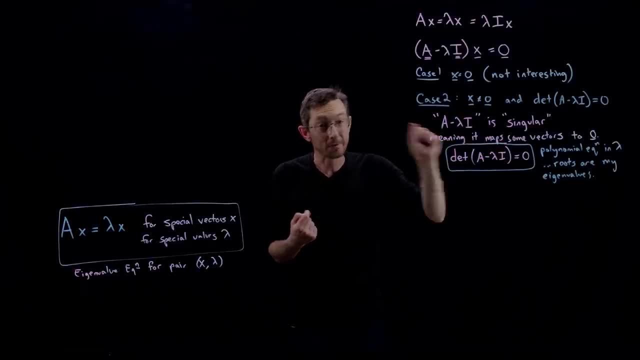 for those lambdas where this is true, for those very specific lambdas, if I have a two by two a matrix, I'll have two of them. if I have a three by three a matrix, I'll have three of them for those very specific lambdas. then there are some X's. 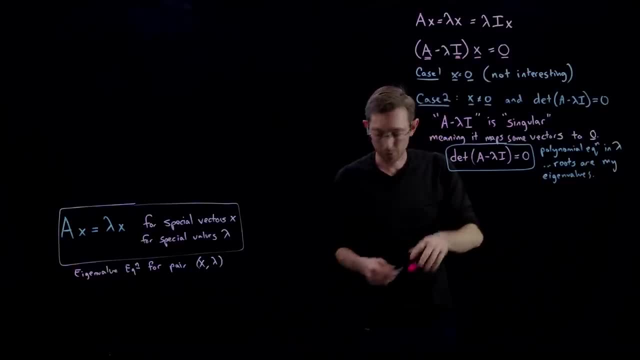 that will map to zero. okay so, and I'll just remind you that this is, in fact, exactly the characteristic equation when we're talking about differential equations. characteristic equation when we're talking about differential equations. okay, good, so I'm just about to. I'll show you how this works on that. 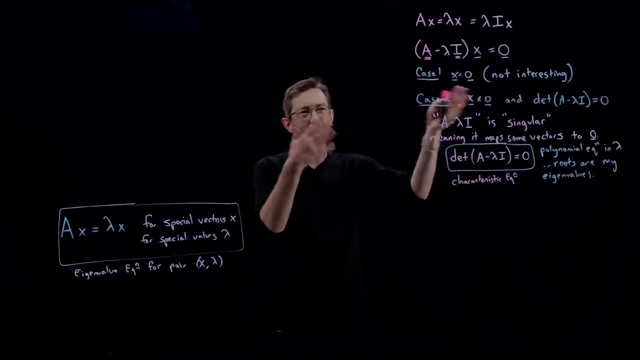 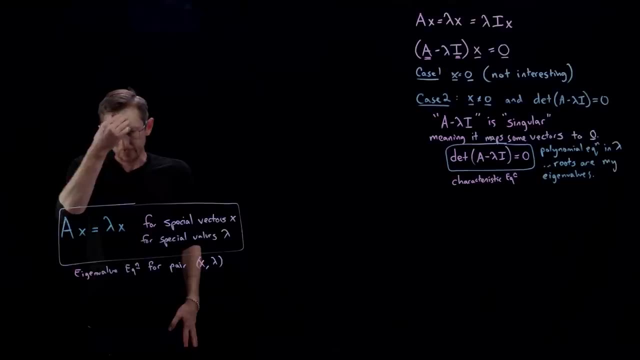 previous example in that two by two system example, but I want to remind you how to compute the determinant of two by two and three by three matrices and things like that. so maybe the first thing I want to show you is that the determinant, the determinant of a matrix, a measures the volume of a square after you map it. 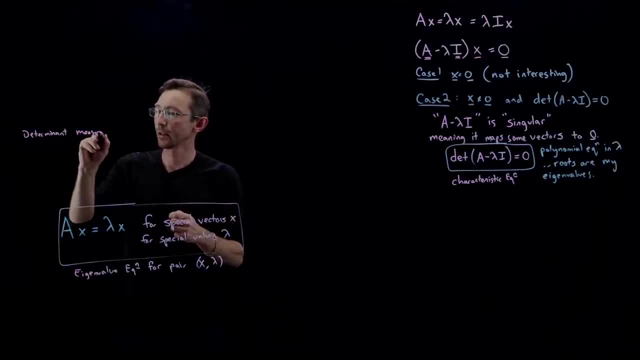 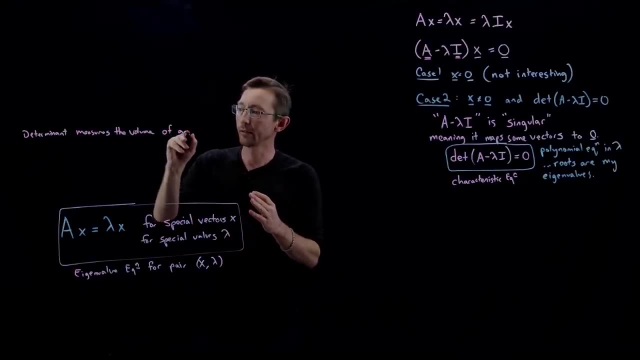 through a. so how do I want to say this? this measures the volume of a unit cube of a unit cube after all of the sides get mapped through a. a the determinant of a matrix. a measures the volume of a square after you map it through a, after all sides are mapped. 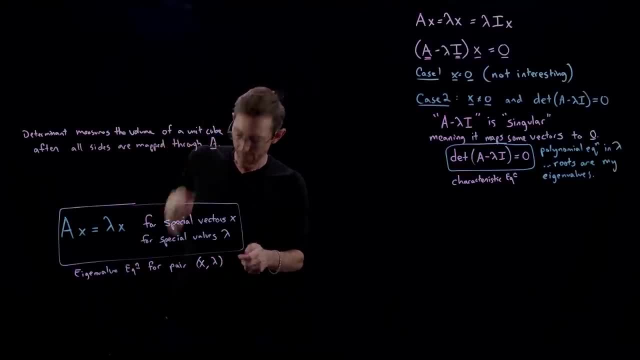 through. I'm gonna draw you a picture, don't worry through a. so specifically, if I take, like this example of a equals two, one one, two, really simple a matrix, what I mean by a unit cube is I literally take a little unit vector in the x1 direction- this is x1- and a little unit vector in the x2 direction and I say: 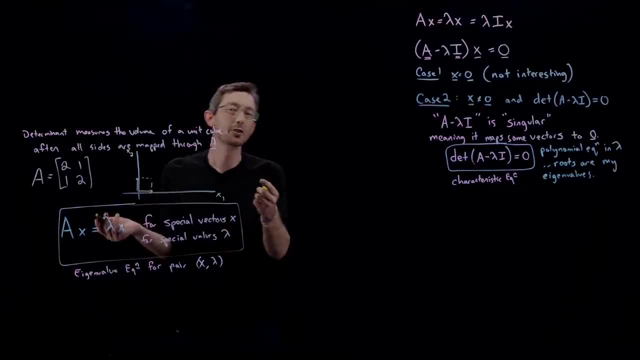 that this is a little. you know, in two dimensions it's a square. in three dimensions it's a cube. in four dimensions it's a hypercube. so I take this you know square in 2d or a cube and nd and I map each of those legs through. 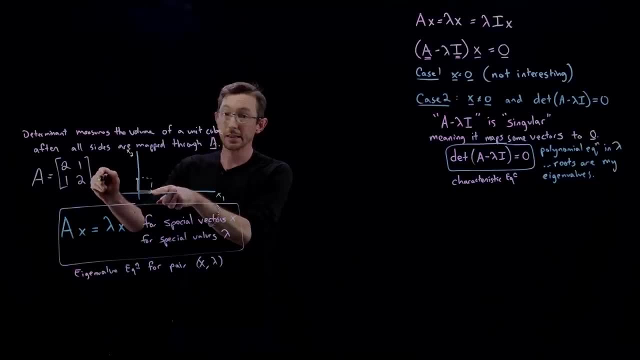 this a matrix. so my one zero leg gets mapped to two one. so that goes from here to here. so this little leg gets mapped here. okay, my this vector gets mapped to here and this little vertical vector zero one, zero one gets mapped to one, two. I take one step over and two steps up and this is that. 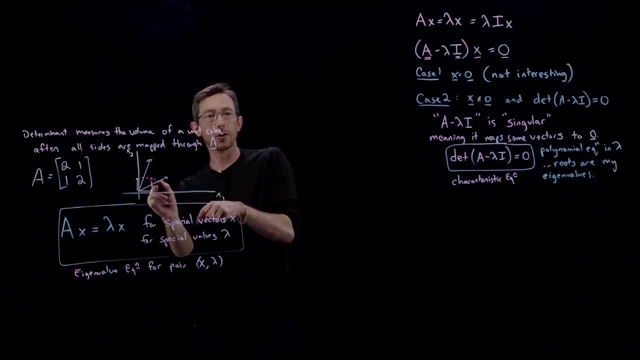 vector there and you could also take this little far corner here and map it through and you'll find that you get this kind of parallel parallelogram and I drew a really bad job of that parallelogram. let's see if I can make this not so horrible, not a. 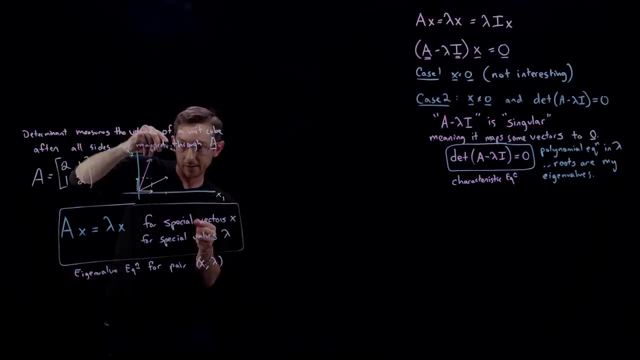 perfectionist but I do have standards. okay, that's better. and so now, if my original unit- skew, square or cube- had area one- because I had length one on all sides- or volume of this pink deformed parallelogram is going to equal the determinant of a, and for a 2x2 matrix like this, the determinant of a is going. 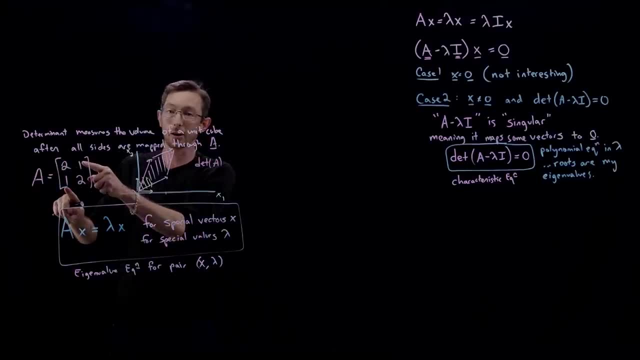 to be the product of the first main diagonal minus the product of the second diagonal. so that's 4 minus 1 equals 3. so the area of this pink parallelogram is equal to 3. it's equal to the area that the determinant of this a matrix, and so 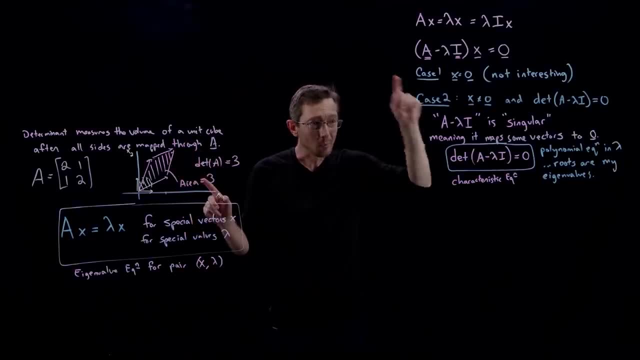 this is kind of how I want to convince you that when this thing has determinant 0, it's singular. it means that I map some directions to 0. what is the only way that I could map these, this little yellow square here, to something with 0 area? the only way I could map it to something with 0 area is if these: 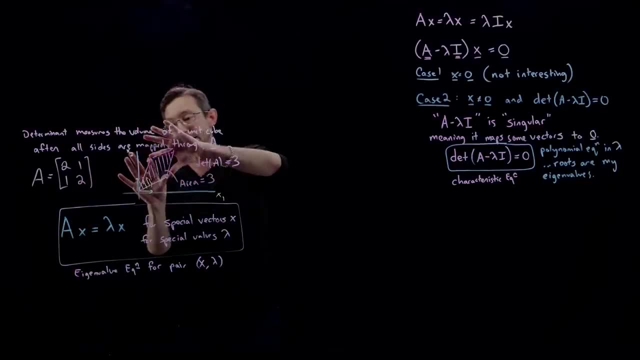 vectors map to something parallel, so this squished together and had 0 area, and what that means is that the only way that these two vectors, this two dimensional space, can map into a one dimensional space with 0 area is if there is some direction that maps to the origin, that maps to 0. okay, that means 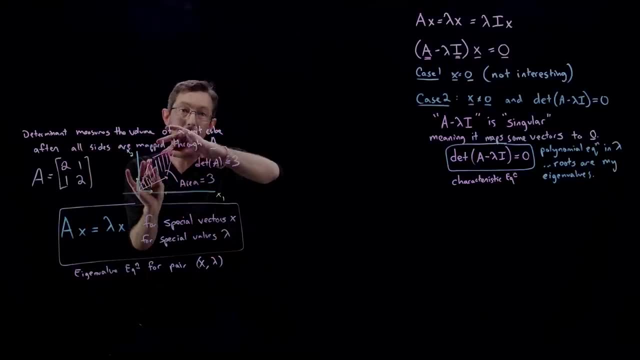 there's some direction that's getting collapsed and kind of smooshed out of this. to give this 0 area, so when my determinant is 0, that means that there are some directions that are being obliterated. obliterated, then a times that direction will equal 0. some directions are getting. 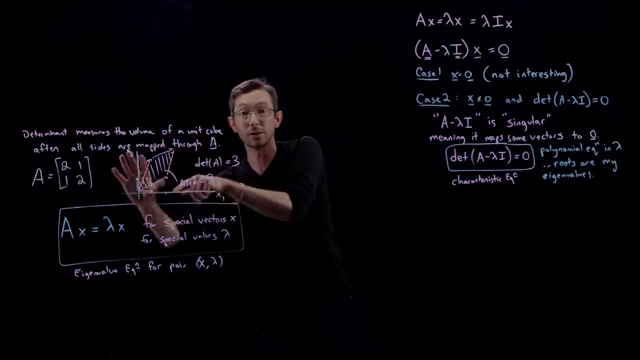 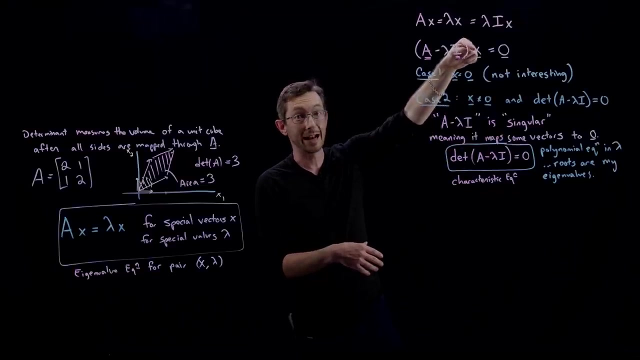 obliterated. I'm losing dimensions, I'm going from two dimensions to one dimension. that's the only way this thing could have area 0 is if it's kind of one dimensional and infinitely thin, and so that's what I mean here when I say that this matrix has determinant 0. there are certain directions, certain X's that get. 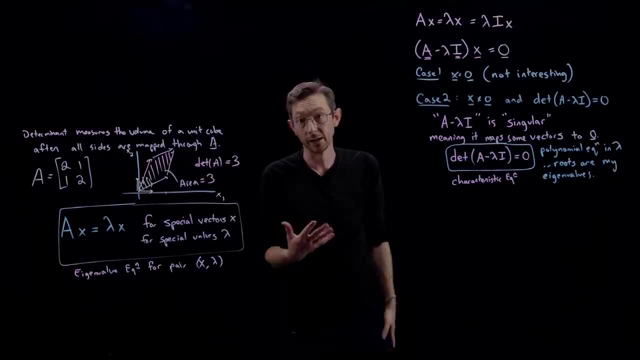 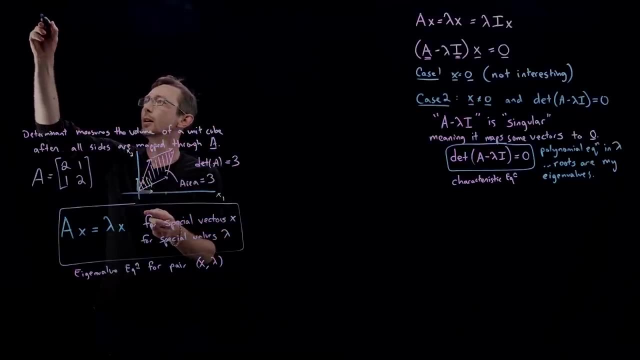 obliterated because this thing has area 0 when the determinant is equal to 0. I'll show you how to take the determinant of a 3 by 3 matrix, because I think that's important for you to know. so, debt of a 3 by 3 matrix when I have, let's say, B 1 1, B 1- 2. 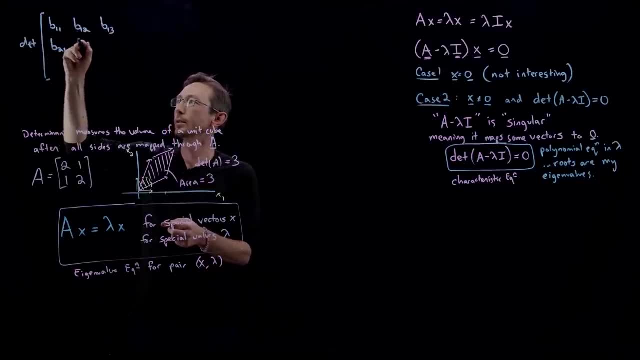 B 1, 3, B 2 1, B 2, 2- I'm gonna stop talking. B 2, 3: I'm not gonna stop talking. apparently okay. so the way you take this determinant is again similar to this one. I'm going to take the first element times the determinant of its the 2 by 2 block, where: 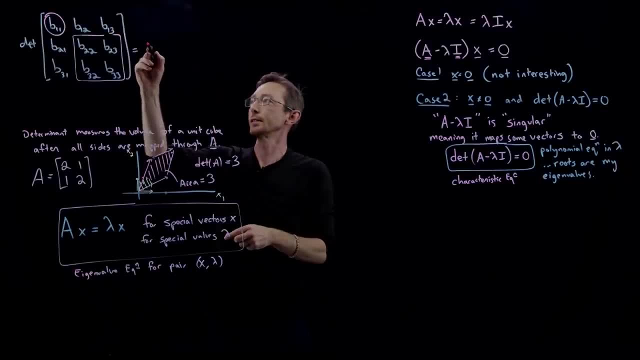 you omit the first row and column that this B 1, 1 is in. so that's B 1, 1 times the determinant of this thing, which is B 2 2. B 3, 3 minus B 2, 3. B 3, 2. okay, there's that one minus. 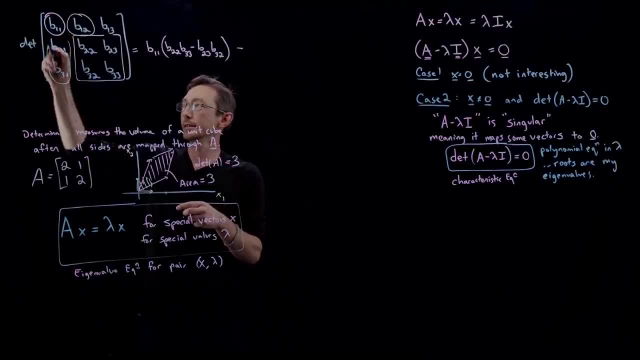 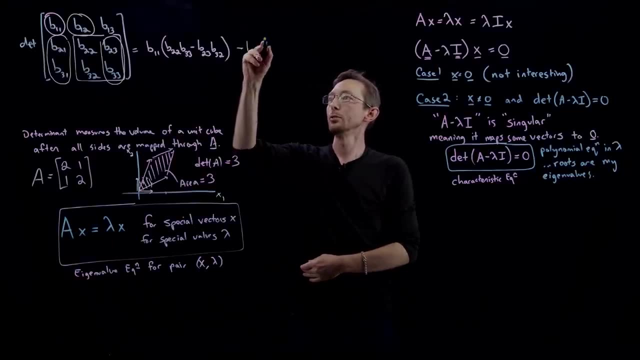 this times the determinant of its sub block, if you omitted that row and that column, so that's B 1 2 times B 2 1. B 3 3 minus B 2, 3, B 3 1 and then finally plus let's. 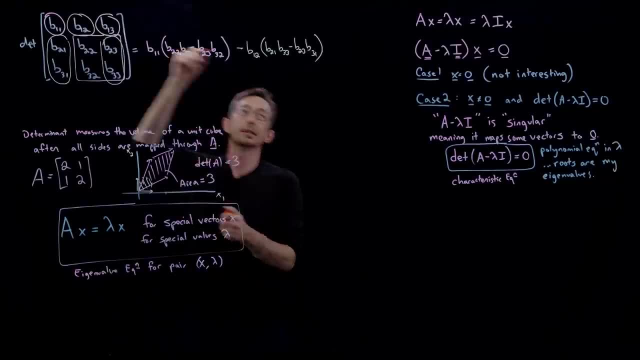 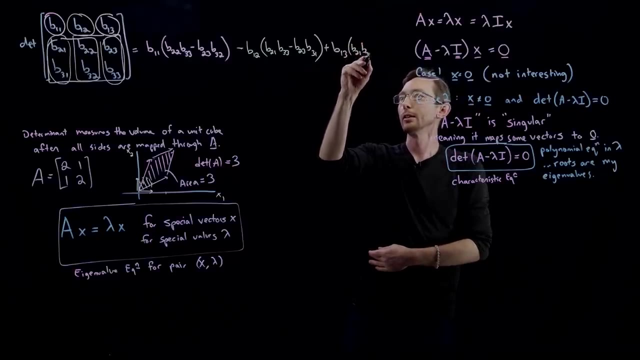 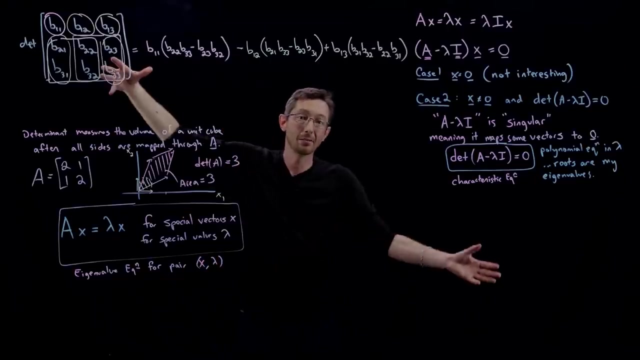 pick a different color, maybe I'll do orange plus B 1, 3 times the determinant of this 2 by 2 sub block that you get when you omit this row in this column, and that's B 2 1, B 3 2 minus B 2 2, B 3 1. okay, and if I had a generic n by n. 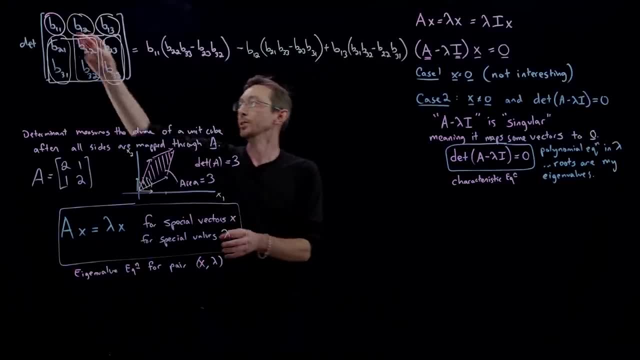 matrix. I do the exact same thing and it's recursive and it's horrible. you take this one times this sub block minus this one times this sub block, plus this one times this sub block, minus this one times this sub block, and then for those sub blocks you'd have to do the same thing recursively and it'd become a 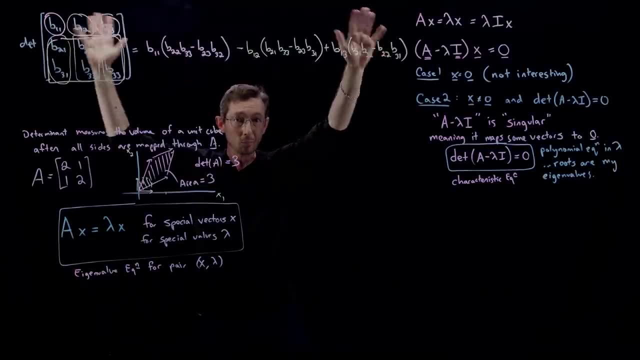 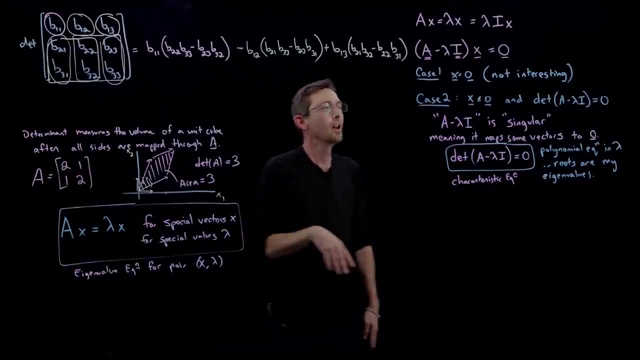 real mess. but this is it for a 3 by 3 matrix and for a 2 by 2 matrix. it's trivial: just product of the diagonals minus product of the off diagonals. okay, so that is what you need. you need to be able to compute these determinants of. 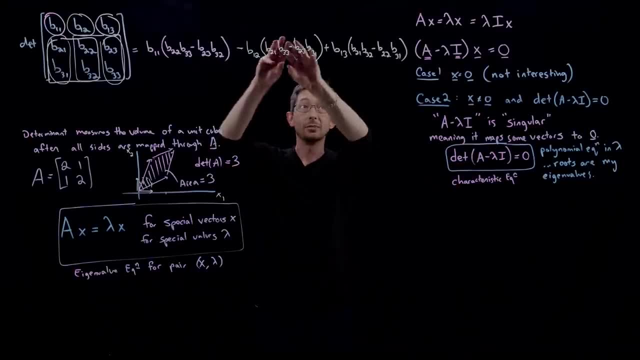 these a minus lambda, I's to get a polynomial. it's going to be some big, nasty polynomial in lambda and then you're gonna solve that polynomial for its roots, the lambdas that make that equal to 0. those are your eigenvalues. then we take those eigenvalues and we take those eigenvalues and we take those. 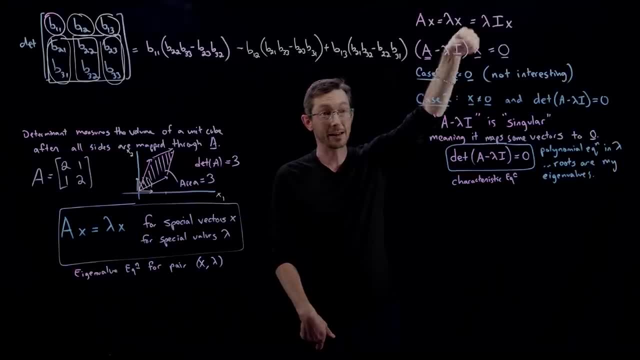 then we take those eigenvalues, and we take those eigenvalues, and we take those eigenvalues, plug them into here and find out which X is get obliterated, which X is mapped to 0. those are your eigenvectors. okay, I'm gonna erase some stuff and then we're gonna do an example, the exact same example we did last time. 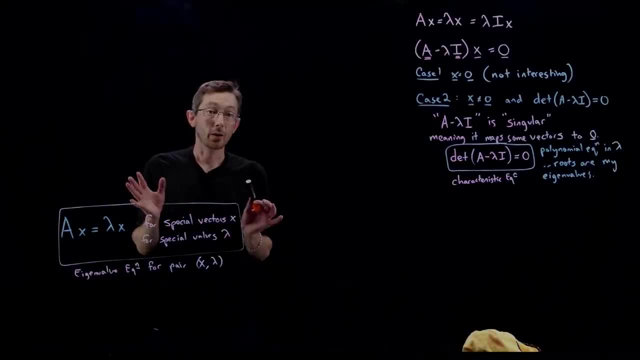 so just stay put. okay, we're going to now solve for the eigenvalues and eigenvectors for that same little 2 by 2 a matrix we worked on before. so our example is a equals. I think it was 3 minus 1 minus 1- 3, 3 minus 1 minus 1, 3. the first thing we do is we compute a minus lambda. 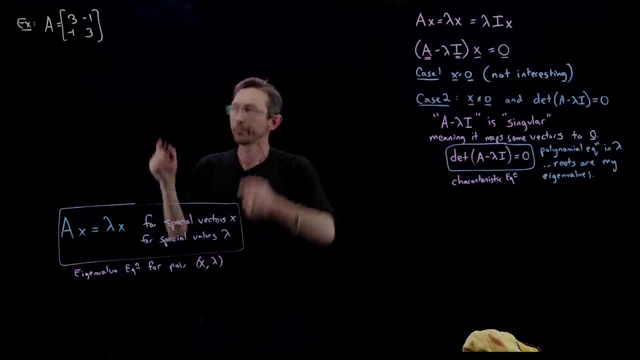 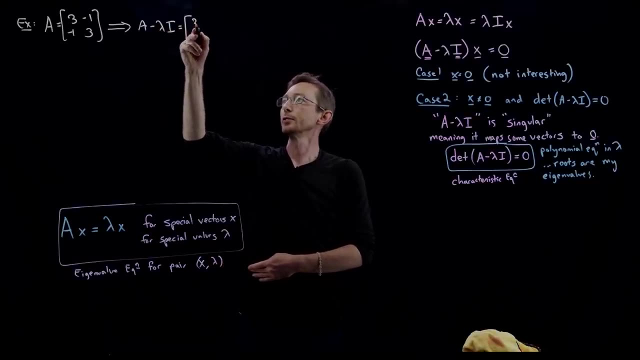 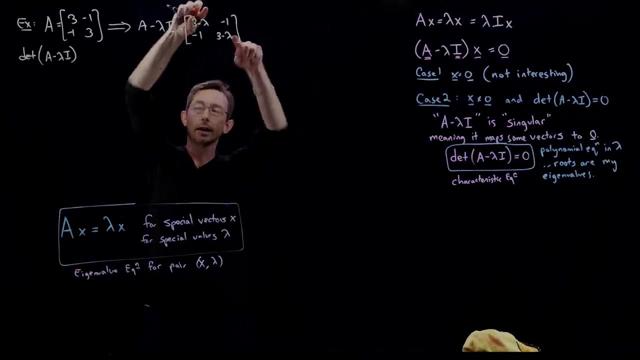 I take its determinant and solve that characteristic polynomial. so a minus lambda times. the identity is easy. this is just 3 minus lambda minus 1 minus 1, 3 minus lambda. taking its determinant debt of a minus lambda, i is just the product of the diagonals minus the product of the off diagonals. so this: 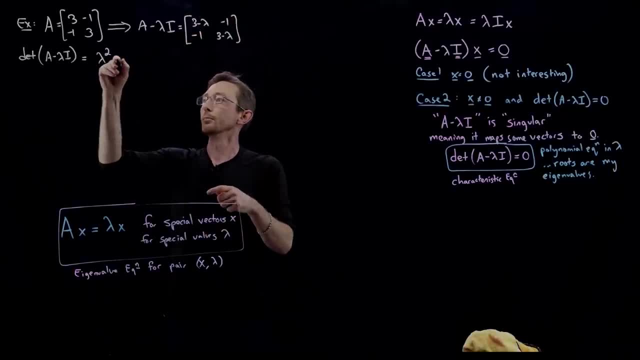 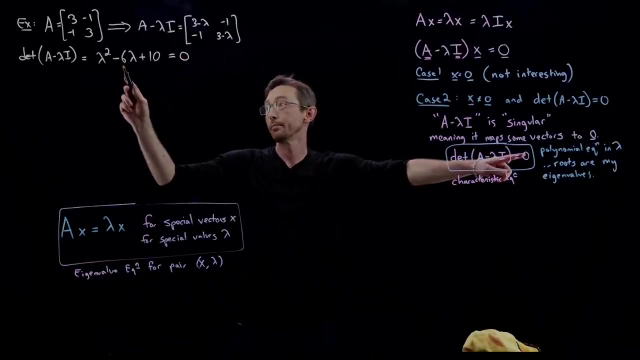 is lambda squared minus six. lambda plus nine, plus another one, so plus ten. just slow down and confirm that that's true. and this has to equal zero for my eigenvalues. and so now you see that this is actually just a simple polynomial equation, so i can, um, did i do this right? 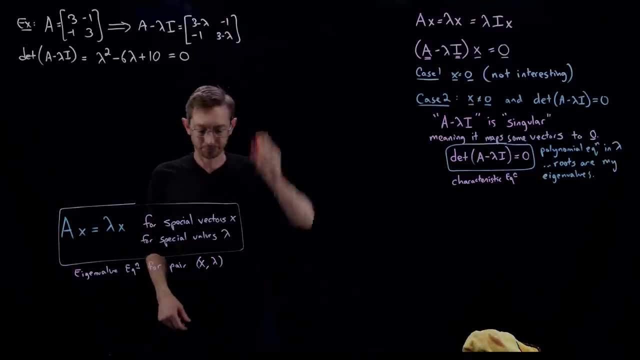 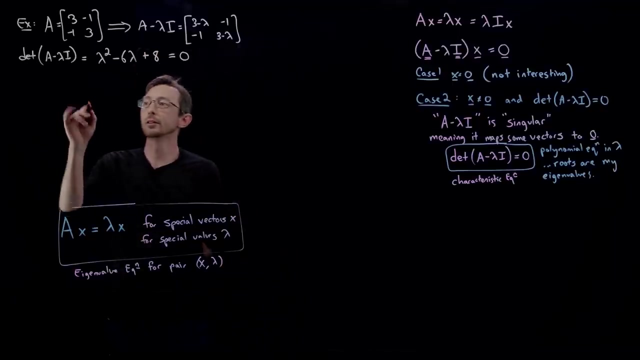 nope, i totally didn't do this right. um, that was nine minus a, plus one, which is minus one, so this should be an eight. okay, that should be an eight. so this is plus eight, and this is going to be a lot easier for me to do in my head. so now i factor this thing and this looks like: uh, lambda minus four. 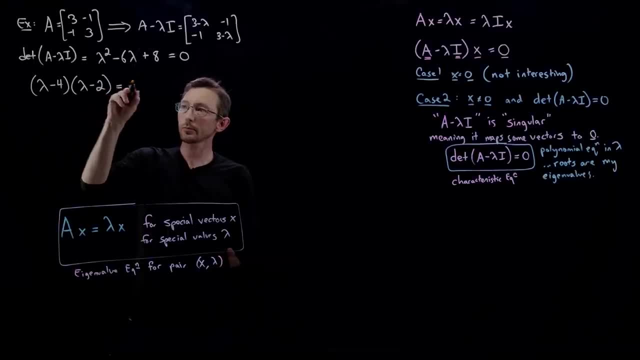 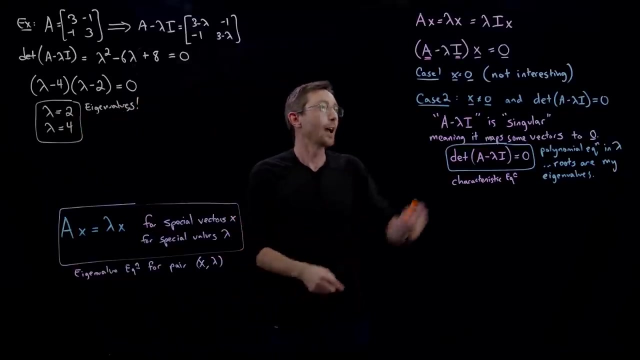 times lambda minus two equals zero. just confirm that that you know. lambda squared minus six, lambda plus eight: good, and so lambda equals two and lambda equals four are my eigenvalues. good, okay, we're cooking with fire. now for lambda two and lambda four. i'm going to find the x that. 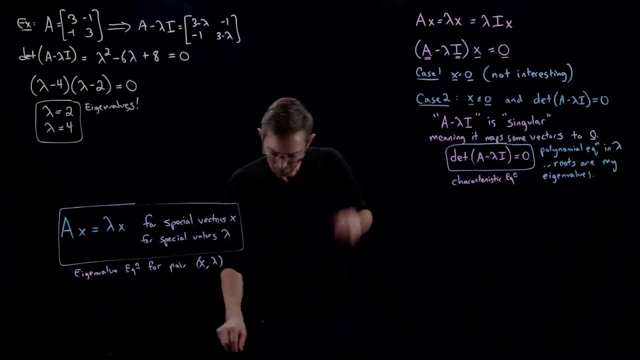 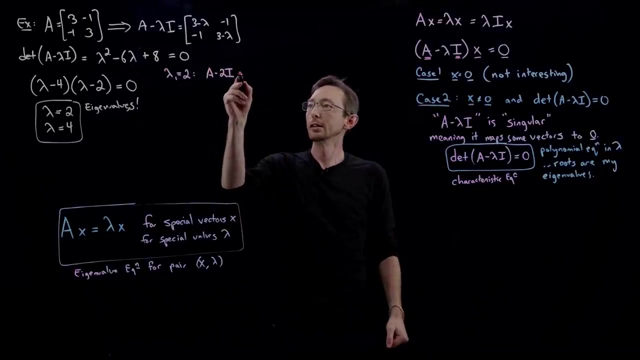 gets mapped to zero. those are going to be my eigenvectors, so this is pretty easy. um, okay, so let's just do this. lambda one equals two. let's start with lambda two. so now i take a minus two i, which is um a minus two. i is just one minus one, minus one one, and i'm trying to find the x vector. 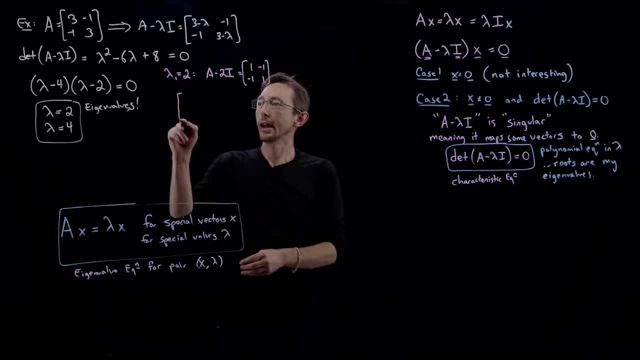 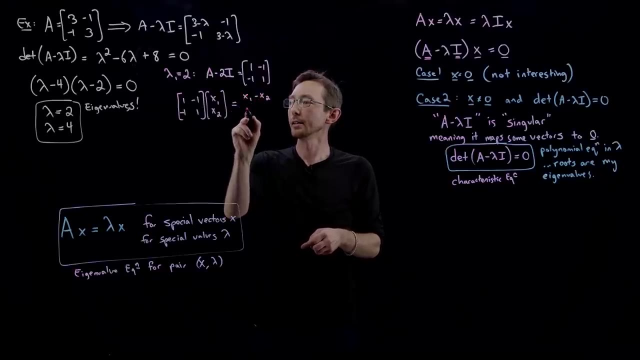 that gets mapped to zero through that mapping. so i have you know, one minus one minus one, one times x1- x2. okay, um, that's going to equal x1 minus x2 and x1, x1 plus x2, and clearly, if x1 equals x2, both of these equals zero. 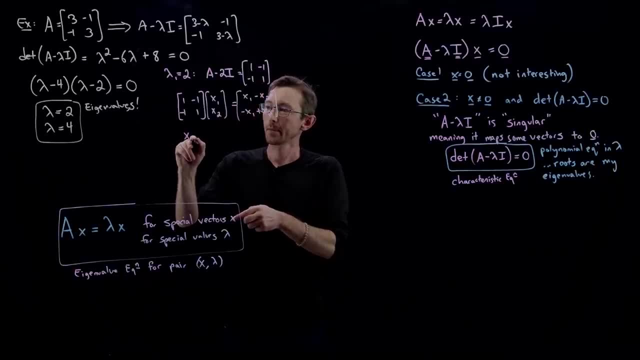 so x1 equals x2. x1 and x2 could just be equal to one one. x2 will be equal. x2 and x2 could just be equal to one one. x1 and x2 could be equal to one one: 1. okay, so that's an eigenvector. I went a little fast, but I think you can convince. 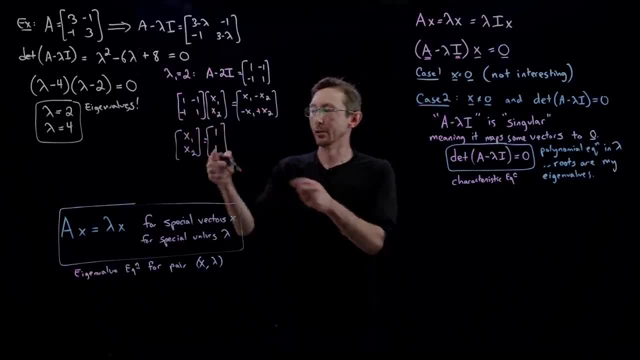 yourself. I tried to find the X that would map. you know, for X equal, for X 1 equals X 2. this maps to 0 if X 1 and X 2 were equal to each other. okay, that's what I do here. similarly for lambda 2: lambda 2 equals 4 a minus lambda 2 minus. 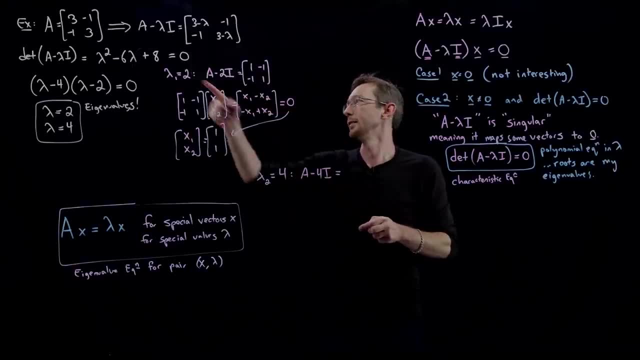 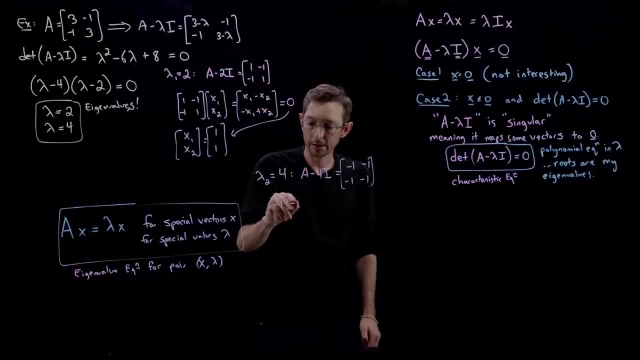 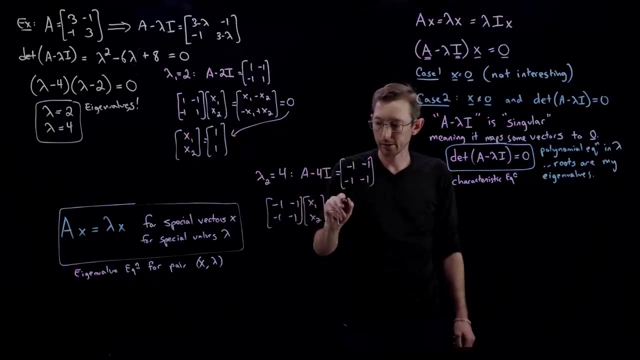 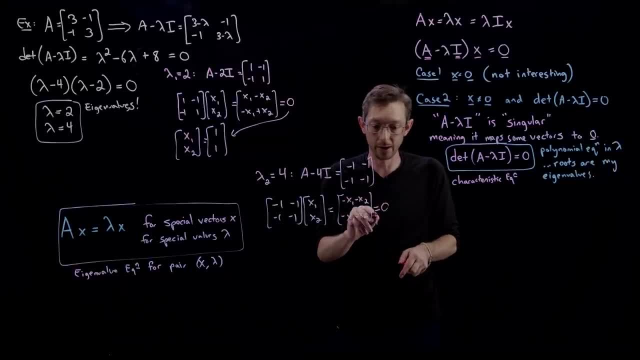 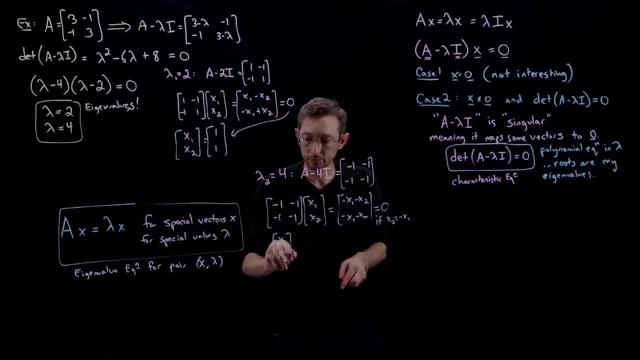 opposite of X 1. both of these will equal to 0. this will equal 0. if you X 2 equals minus X 1, and so I can say that X 1 X 2 equals. you know, 1 negative 1 is an eigenvector, so this is an eigenvector corresponding to lambda 2.